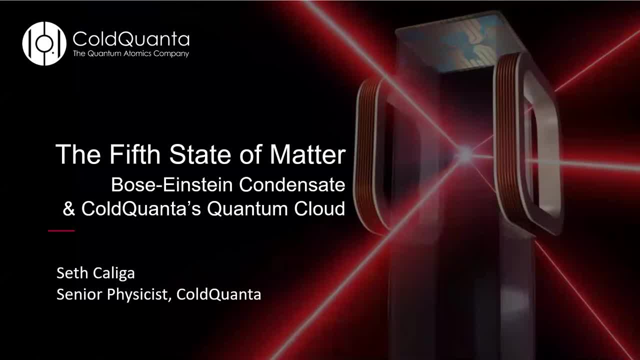 about Bose-Einstein condensation, a phenomenon that's sometimes referred to as the fifth state of matter, and for me to give you a peek at some of the exciting services that Colquhanna is going to be rolling out shortly to folks like you. 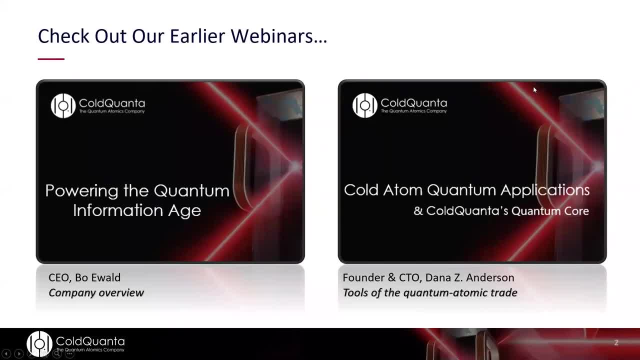 So first I'd like to take a moment to point you towards our first two webinars, if you happen to miss them, And the first was given by our CEO, Bo Ewald, and provided an overview of Colquhanna's mission. The second was actually given by 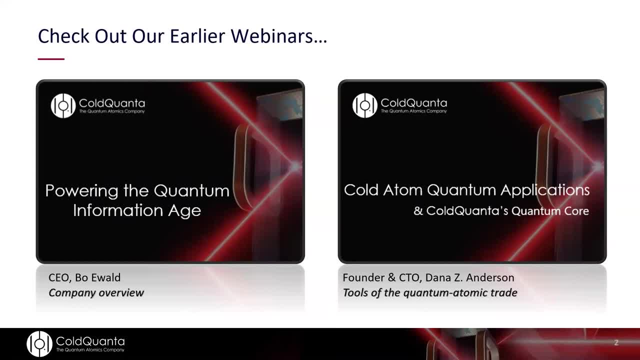 our founder and CTO, Dana Anderson, who covered some of the amazing tools that we use to control our quantum of choice, which is neutral atoms, And both of these events are available to you from the events page on Colquhanna's website. I encourage you to check them out. 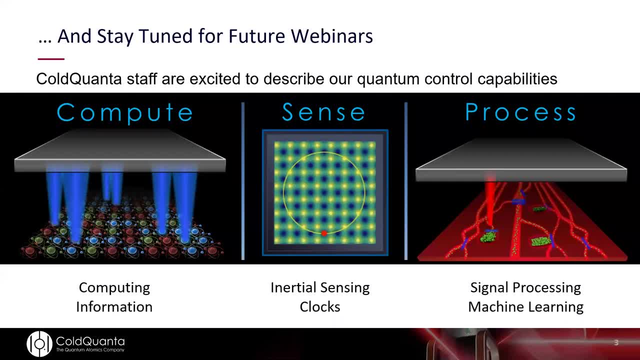 I also hope you would stay tuned for the webinar series that follows this one, which continues to dive deeper into the services that Colquhanna looks to provide our customers across three major thrusts. That includes computing and quantum information, sensing and timekeeping. 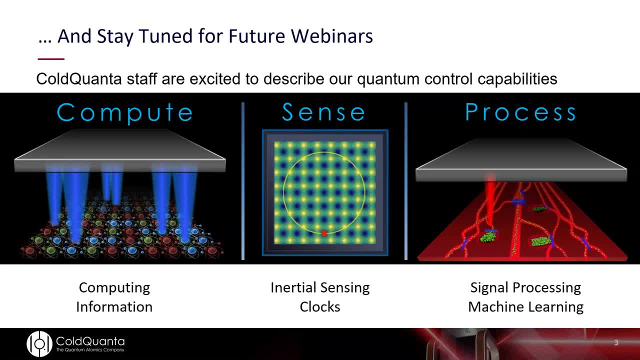 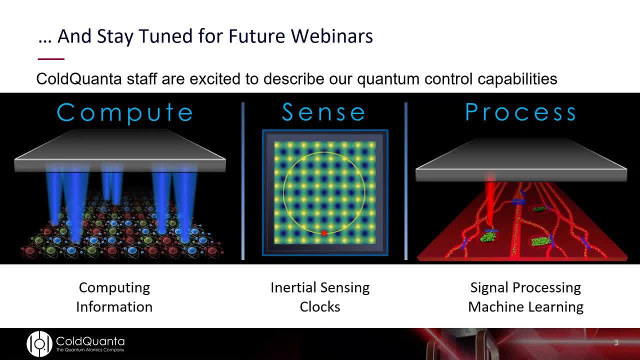 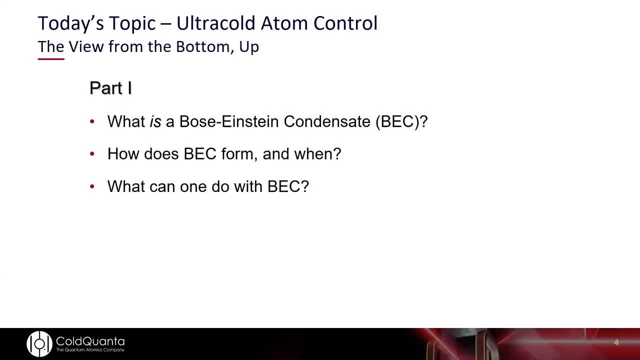 interesting things like quantum machine learning, that we're working towards, And our staff, many of us- are eager to continue digging deeper into these topics, telling you, our customers and general audience, more about them. So, getting to today's main event, I'm going to tell you a little bit, kind of from. 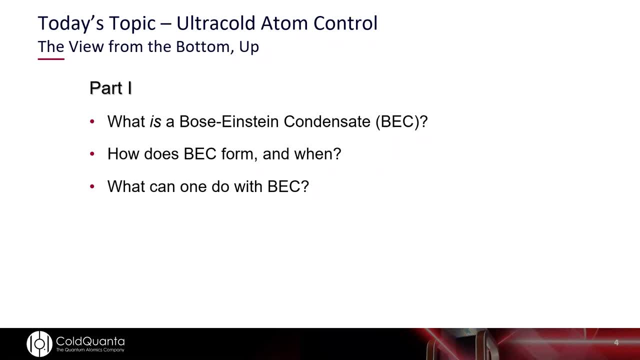 the bottom up perspective about ultra-cold atom control. I'll start by describing what a Bose-Einstein condensate is- We call it BEC for short- and what it isn't. more importantly So, we'll also go into how and when BEC is formed and also what useful things we can do with them. 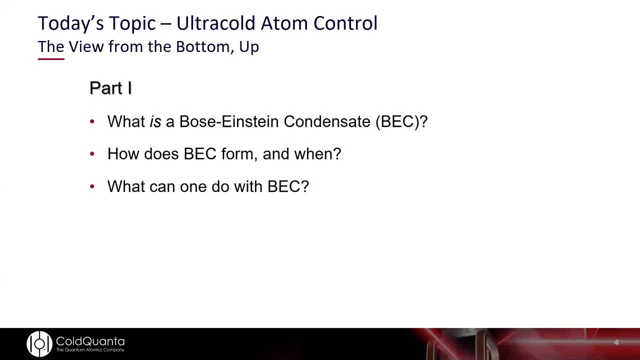 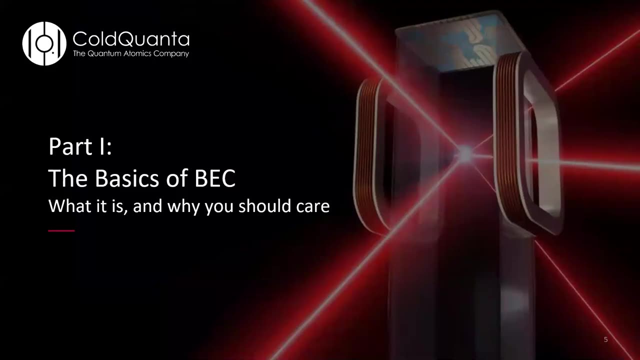 After all, hopefully, there's something useful for them. And in the second half I'll introduce a project that we finally dubbed Albert and tell you how folks like yourselves can experiment with Bose-Einstein condensates. All right, jumping right in. let's begin with some of the basics of BEC. 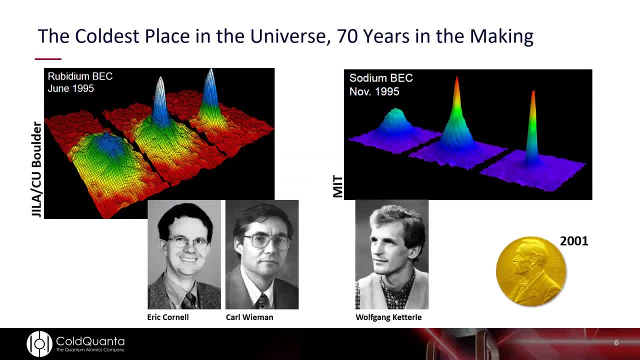 Right. so what is Bose-Einstein condensation? If you've heard of it before, you may have seen these pictures and probably have heard of these folks at the bottom of the screen. The images at the top are actually some of the first snapshots of the original Bose-Einstein. 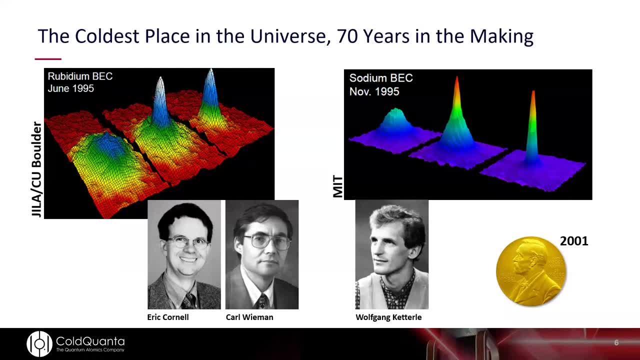 condensates that were ever created. On the left, we have some that were made in June of 2020.. These are some of the first snapshots of the original Bose-Einstein condensates that were ever created. On the left, we have some that were made in June of 2020.. 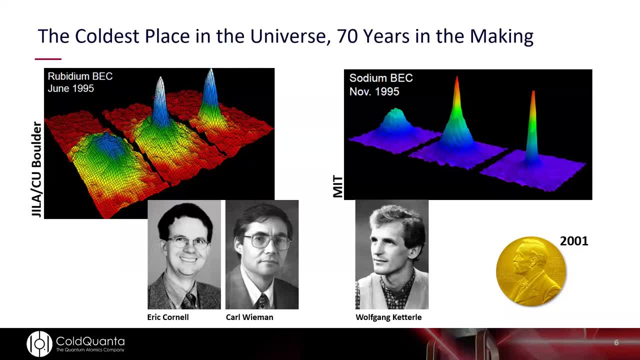 And on the right we have some that were made in June of 2020.. These are some of the first snapshots of the original Bose-Einstein condensates that were ever created, And on the left we have some that were made in June of 2020.. 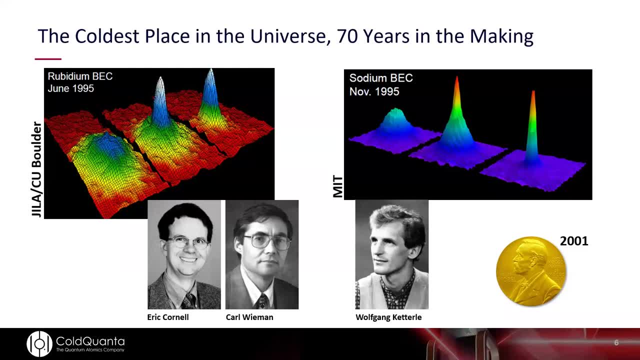 And on the right we have some that were made in June of 2020.. And these were condensates of rubidium atoms. And shortly thereafter, researchers in the group of Wilk and Kelly at MIT also achieved BEC, and this time using sodium atoms. 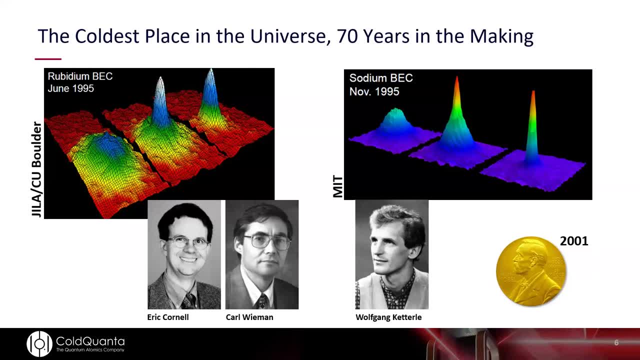 So what are these images? Well, they're the canonical triplet of three false-colored images, And they're taken moments after the atoms have been released from an electromagnetic trap that is surrounding and confining atoms in an ultra-high vacuum chamber In the system. it really takes these sorts of techniques to sufficiently isolate the atoms. 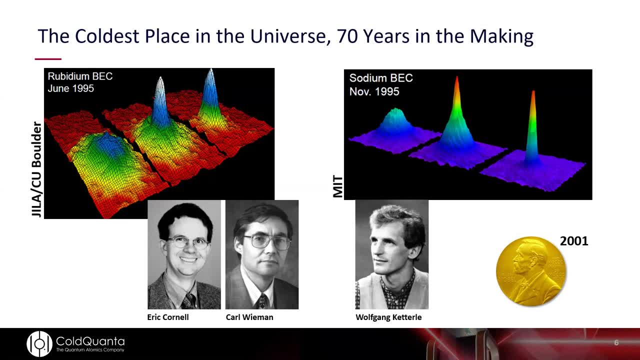 who are now at a temperature less than a millionth of a degree above zero, And also they're surrounded by room temperature objects, so we have to isolate them from those, And these images actually scan through the phase transition of a vapor of thermal atoms. 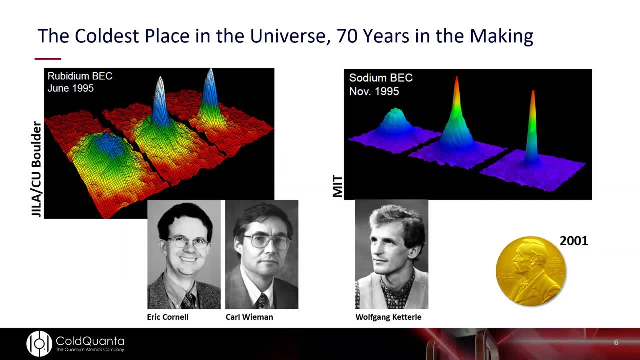 which appears as a broad Gaussian shape to the Bose-Einstein condensate, which starts peaking up at a much higher density Now. Eric Carl and Wolfgang were awarded the 2001 Nobel Prize for this pioneering work in BEC. 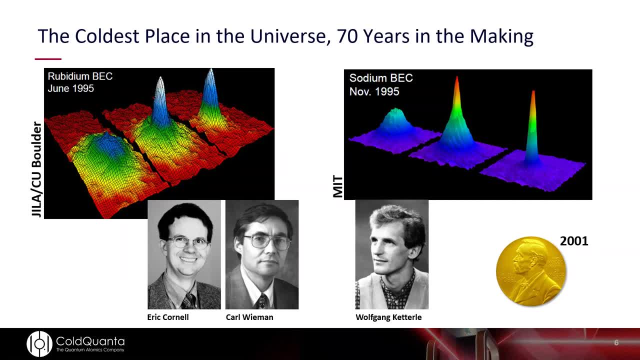 And since then there have been many dozens of academic groups around the world who now routinely make this interesting quantum state in order to study fundamental phenomena. So later this talk I'm going to continue that thought and describe what we at Cole-Kwana have planned. 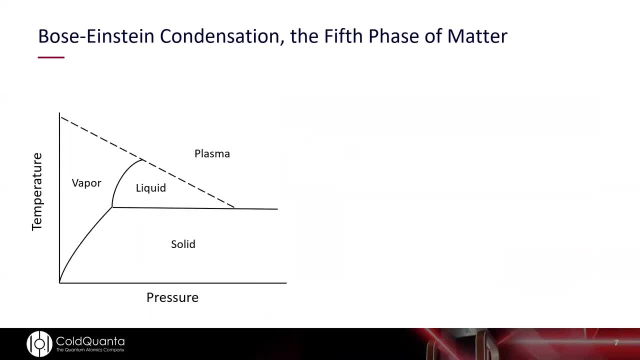 for this interesting state of matter. But first I'd like to clarify a little bit about what Bose-Einstein condensation is and dispel some notions about what it isn't. And I'll start with this generic phase diagram, which many of you may or may not be familiar with. 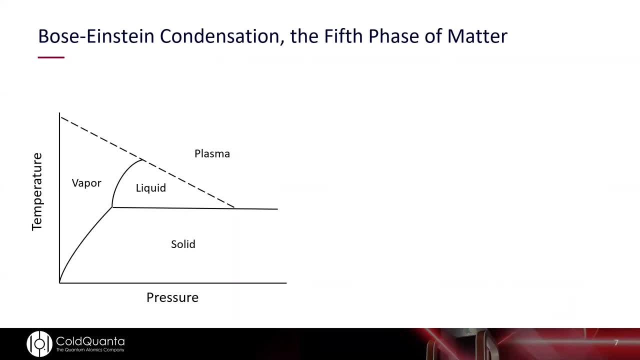 But a phase diagram is actually a useful tool to understand the state of matter And how a single type of matter, whether it be atoms, molecules, what have you? how they behave across different circumstances. So this is a plot of the different phases across ranges of temperature and pressure. 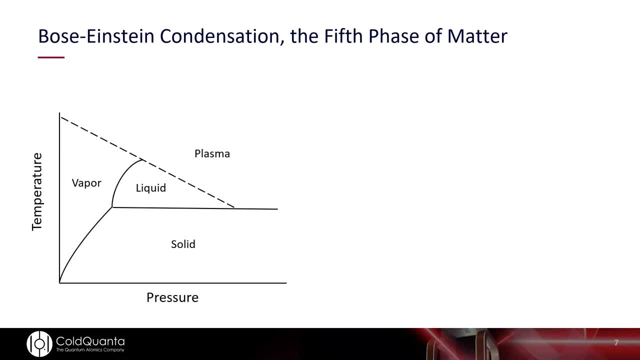 And so from what I've drawn here, you can see that substances exist in a solid form at low temperatures and across a range of pressures, And as that temperature increases and across intermediate ranges of pressure, that material would then become a liquid, And at even higher temperatures and at lower densities, that becomes a gaseous vapor. 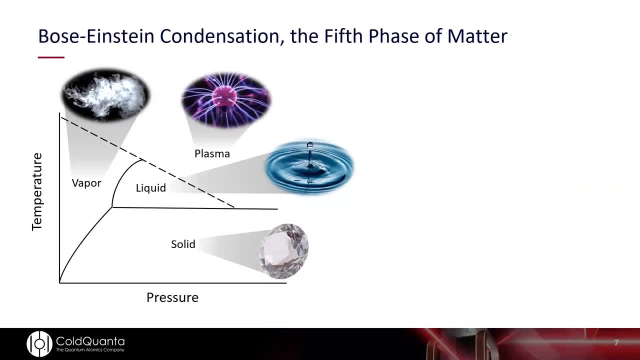 Now we also have the fourth phase of matter, which is a little bit more exotic. It exists around us. you know lightning. You can buy little toys like this from the store that generate plasma. But this happens when the temperature is high enough or energies are high enough to liberate electrons. 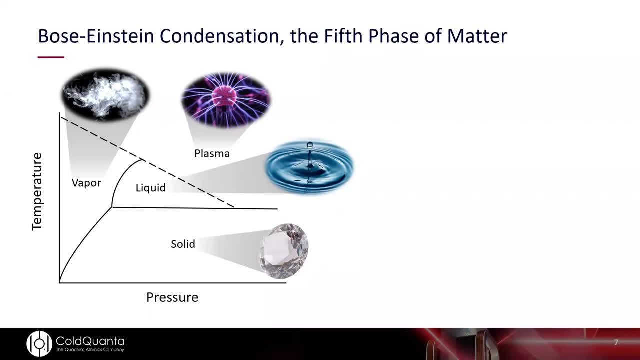 ionizing particles, And that's when the energy is high enough to liberate electrons. And that's when the energy is high enough to liberate electrons, And that's when the energy is high enough to liberate electrons. And beyond these four phases of matter, there's actually interesting dynamics that you can view. 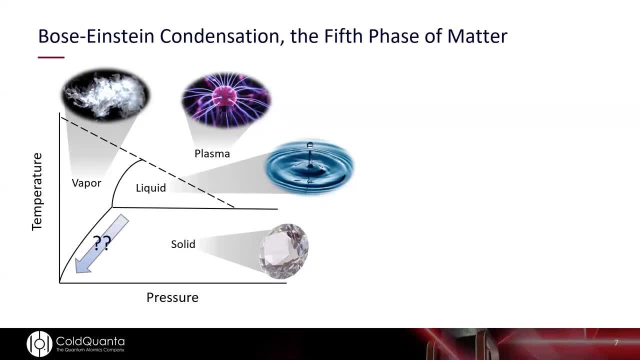 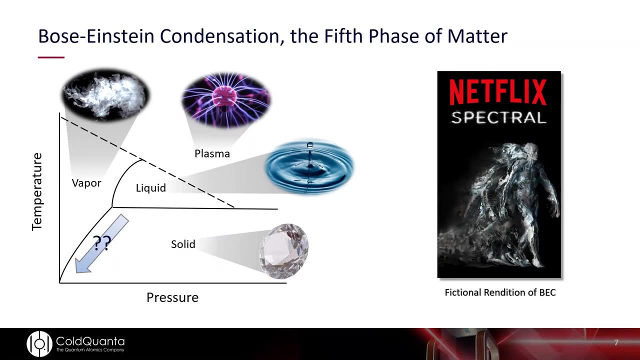 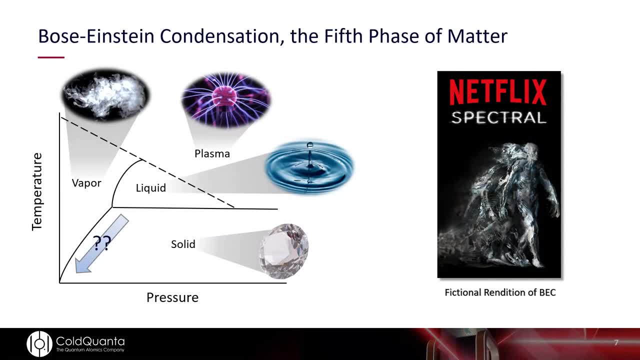 So, whether you've seen it or not, recently BEC has hit pop culture and gave us a little bit of an interest in it. So, whether you've seen it or not, recently BEC has hit pop culture and gave us a little bit of an interest in it. 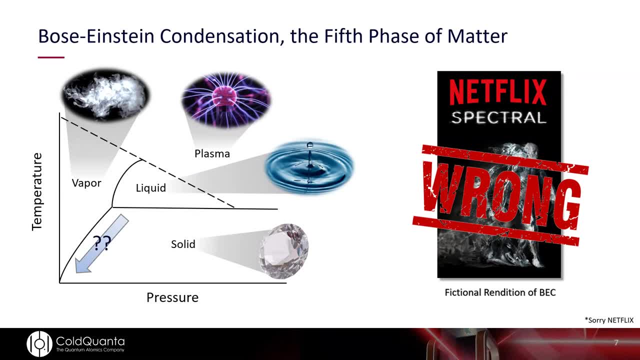 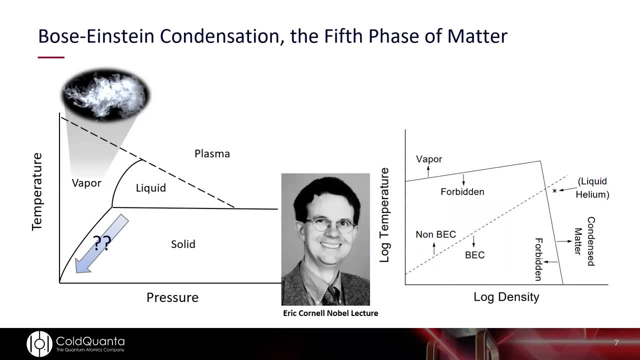 publication to this type of physics, but it also does it a little bit of disfavor. So let's actually take a step back and remap this useful phase diagram to the one that Eric Cornell actually gave during his Nobel lecture, and it's now looking at these things on log scales, so temperature and 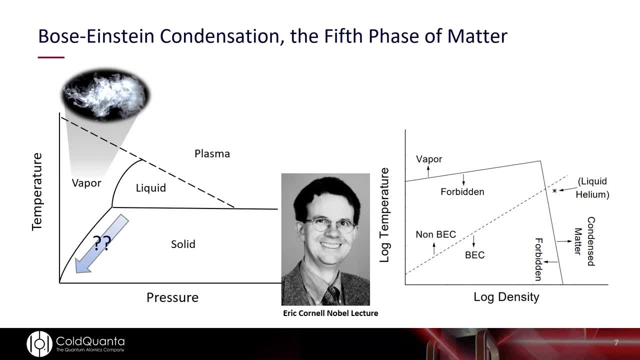 density and it really helps elucidate a little bit what this phase transition to BEC actually is. and usually, if you, if you look at this, you you see that there's this region in here that I've highlighted, where it says BEC, and then there's some different lines going to condense matter. 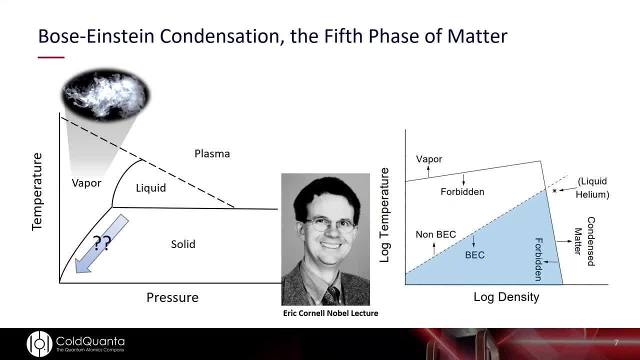 at higher densities, vapor at higher temperatures, but that is to say, above this dashed line, the system has too much energy to condense and above a certain density, the we actually get the material to solidify before it realizes that it's going to condense. So we're going to condense the 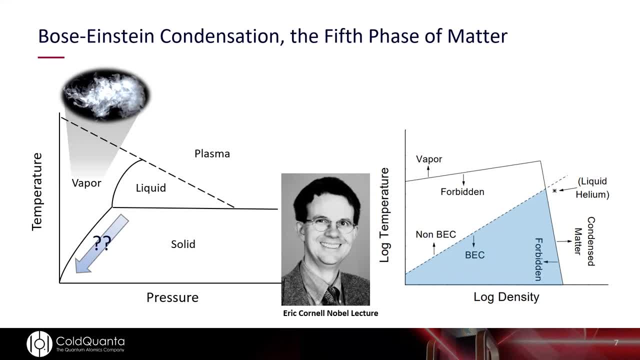 material and then we're going to get the material to solidify before it realizes any interesting quantum behavior. Now, unfortunately, the the region that's highlighted here is in this region where it's actually forbidden by the laws of thermodynamics. but ultimately, if you follow a 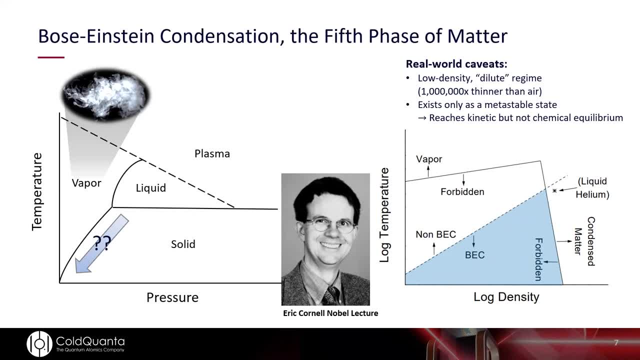 couple real world caveats. you can actually access this region of the phase space diagram and reach boson and condensate. So what that means is we have to have some sort of dilute sample, and dilute in this case means roughly a million times more than what we have in this case. So we have to. have some sort of dilute sample, and dilute in this case means roughly a million times more than what we have in this case. So we have to have some sort of dilute sample and dilute in this case. So we have to have some sort of dilute sample and dilute in this case. So it's gonna be a million times thinner. 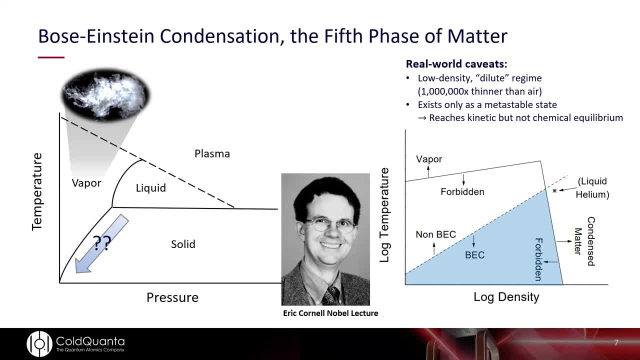 than the air we're all breathing right now, and it's also very cold. And even if we were to reach this boson sine condensate, it's never actually a equilibrium state. It reaches some sort of kinetic equilibrium, but not chemical equilibrium. So even though this is forbidden, we can reach this. 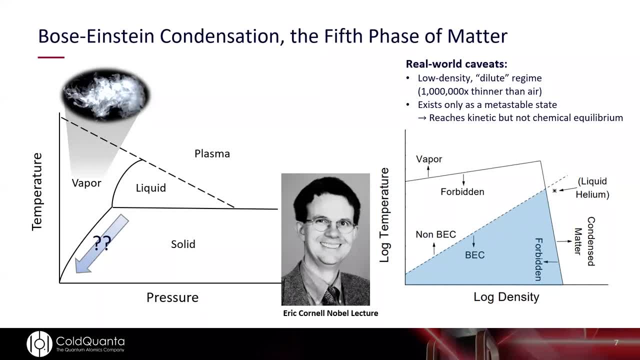 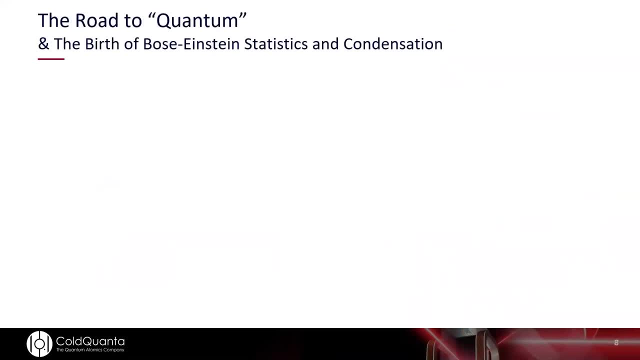 this portion of the phase space diagram and the BEC can exist for a moment in time. So before, Before I tell you how to reach this metastable state, I think it's actually useful to recall the series of discoveries that led to the prediction of Bose-Einstein condensation. 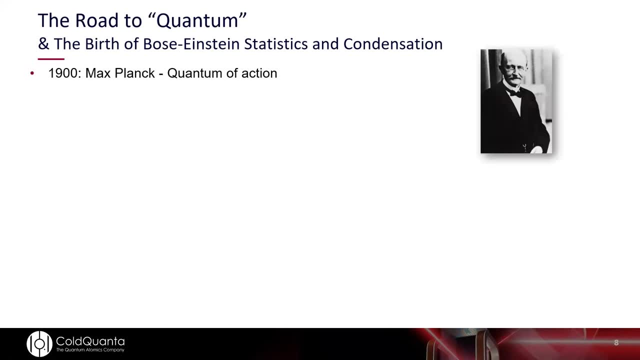 It started over a century ago with Max Planck, and at the time he was actually tasked with a somewhat menial task of actually finding a way to increase the efficiency of light bulbs, which we're all still trying to do to this day, And without getting into the details, it's actually his research in blackbody radiation. 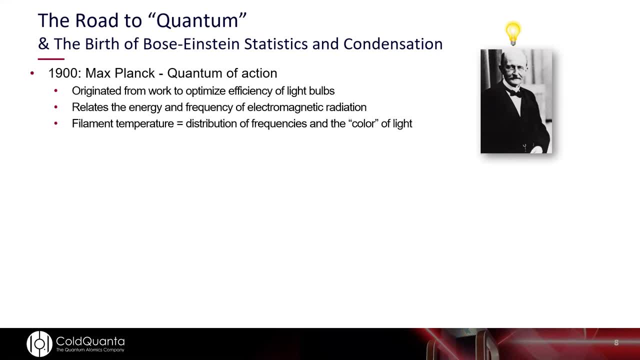 that concluded that a certain color temperature would actually yield the most energy in the visible portion of the electromagnetic spectrum And, indirectly, this realization led him to conceptualize what we call the quantum of electromagnetic action, which relates the energy of electromagnetic waves to its color. 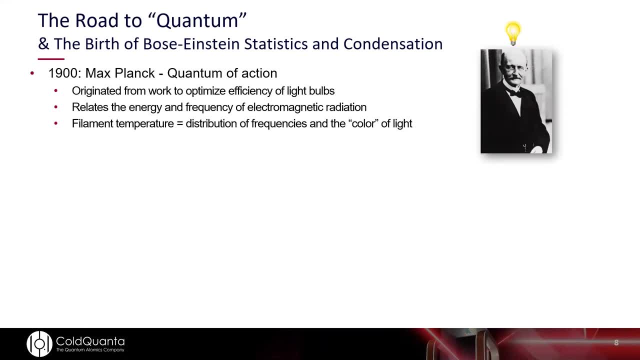 And with this we actually gained a lower bound for the single quantized energy that can exist, And it's astronomically small. It's six times 10 to the minus 30.. 34 has units of joules per hertz, or energy for frequency. 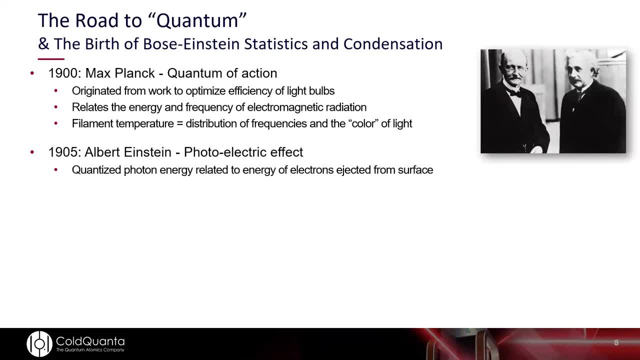 And it's aptly called Planck's constant. Now, shortly thereafter, Albert Einstein. he was working on many things at this time, but one of his most important, and one of his most recognized, was his proposal for a somewhat radical concept which, rather than energy being carried along by a wave, in fact that. 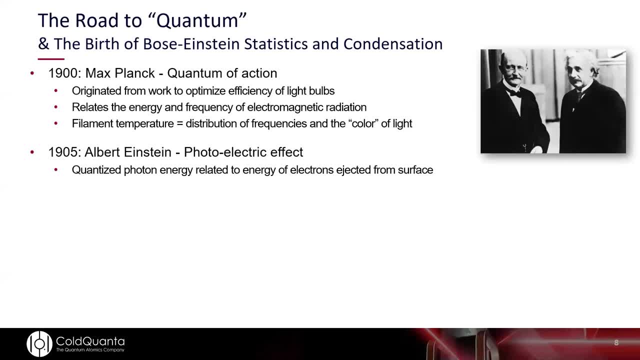 energy is manifested in a wave. It's a wave. There's a packet of energy which was later coined to be photons, And he used this concept to describe the liberation of electrons from metallic surfaces through the application of certain colors of light where that photon energy exceeds. 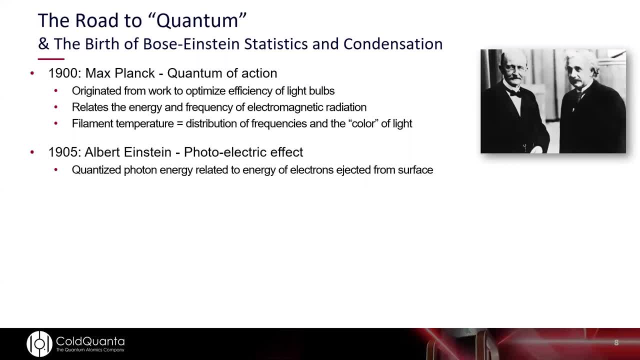 the work function of metal. So you have this: quantized photon comes in, It has enough energy And it liberates a single electron. And without going more into the details on that, we can shift to maybe two decades later, where Satendra Bose, who embraced this, 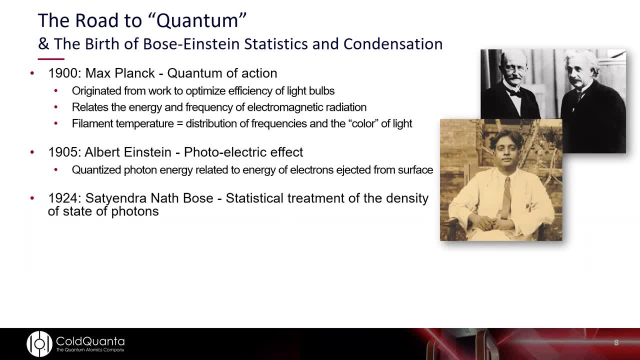 theory of photons, sent Einstein a preprint that actually outlined a statistical treatment of photons and their density of state And, importantly, Bose applied this concept of phase-based density to derive the distribution of photons with respect to their energy and, using this rather simple approach, he was 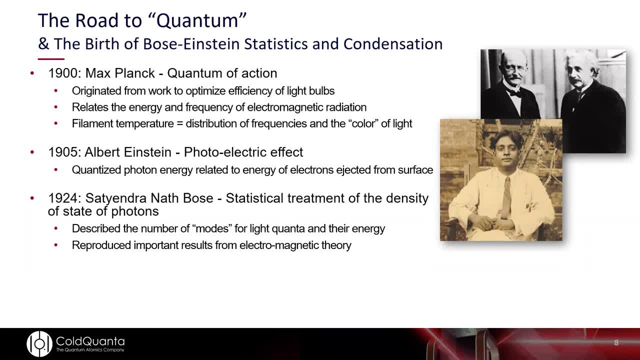 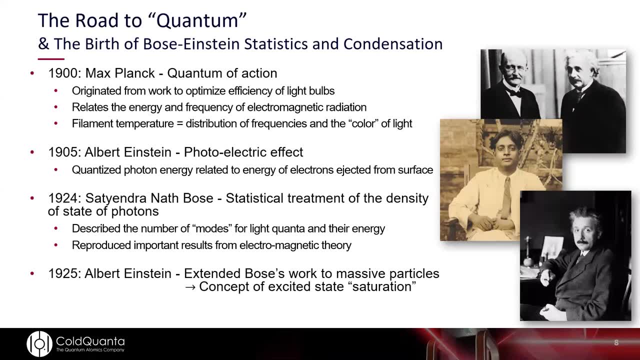 able to reproduce the important results of electromagnetic theories. So all this brings us to this point in time where Einstein was really stimulated by Bose's work, and eventually Einstein extended that theory to massive particles, and so now, rather than having an electromagnetic wavelength, these massive particles have corresponding de Broglie wavelengths. Dana in his past. 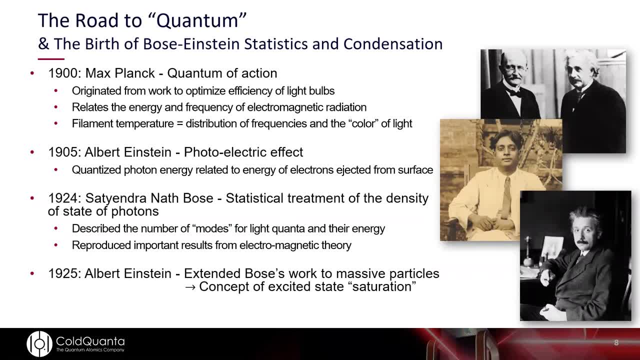 webinar spoke about what de Broglie wavelengths were, And because of this extension and what he published in the paper, he was able to find a way to determine the energy state of these particles. And so what he did was he published over a series of papers- it actually included this important concept. 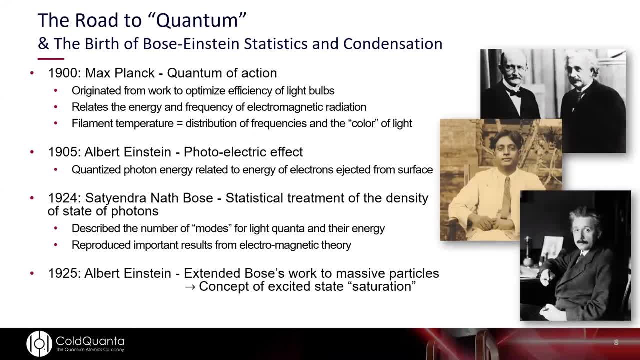 of excited state saturation and this concept, which limits the number of particles that could occupy excited states and, as a result, the remaining particles collapse to the lowest energy state of the system. That's, that was the important moment, and for this to occur, the system has to reach a sufficiently 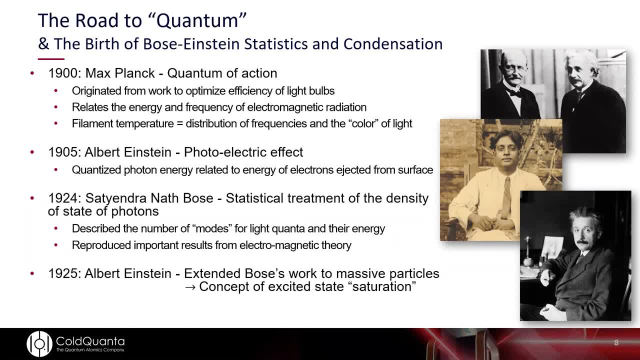 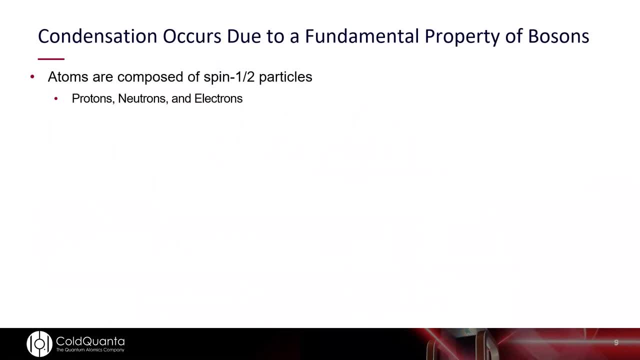 high phase-based density. In other words, it has to be both cold and dense. We now call that collapse condensation. Now I'd like to dwell on this important concept for a moment. So condensation occurs in part because of temperature and density, but 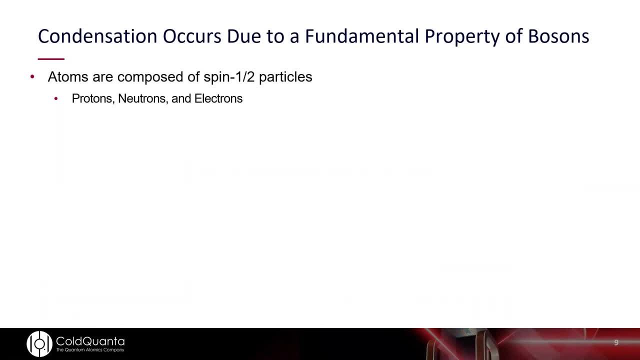 it also. it also occurs because of a fundamental property of bosons, and this includes photons and certain types of atoms. Now, all atoms are composed of three types of subatomic particles- protons, neutrons and electrons. And each of these parents. 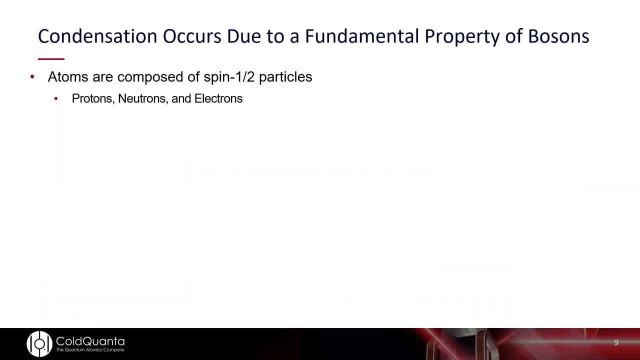 particles carries one half unit of spin and without getting into what the details of spin, atoms with an integer number of these particles have an, even have an integer spin, and these are called bosons and the various energy levels that you can see here on the right in this kind of 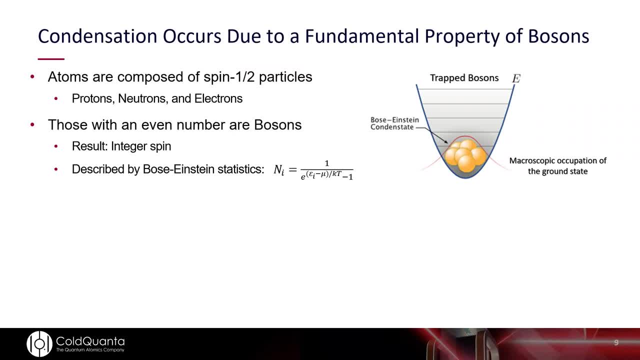 parabolic potential are these different energy levels that particles can exist in and, of course, as I just said a moment ago, if you're cold and dense enough, they reach this macroscopic occupation of the ground state. now, fermions are completely different. on the other hand, where? 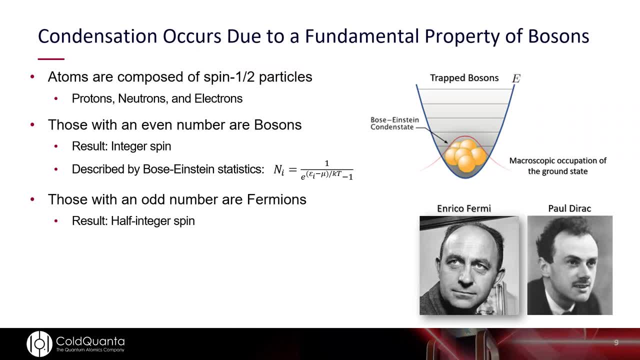 they actually still maintain a half integer spin, and these are named fermions after their the person who discovered them, Eureka Fermi, and in fact it was Fermi who set a different sort of statistics that were later outlined by he and Paul Dirac, and it carries. 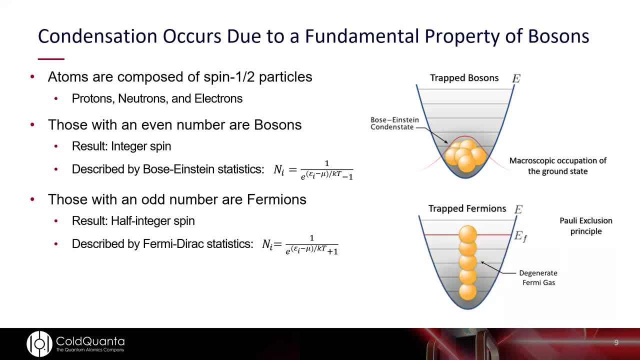 their name. so the these Dirac Fermi statistics, different from the Bose-Einstein statistics, and in turn we see that the atoms now behave completely different in this potential. I'm showing on the right where you have a maximum of two particles that can occupy given energy state. one was spin up and when the other was spin down, and this notable 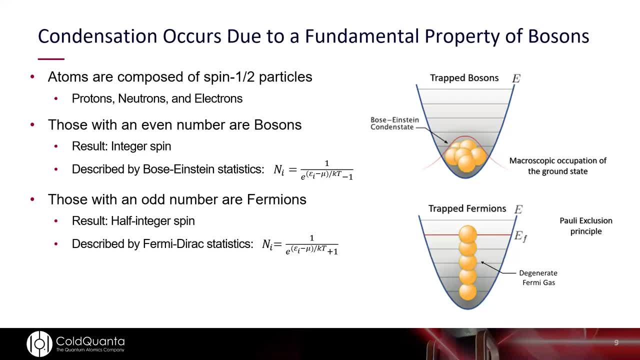 exclusion is called the Pauli exclusion principle, so you can only have two particles in each state and this system fills up until the particles reach the Fermi energy. this sort of behavior also happens in metals with the electrons occupying up to the Fermi energy level and 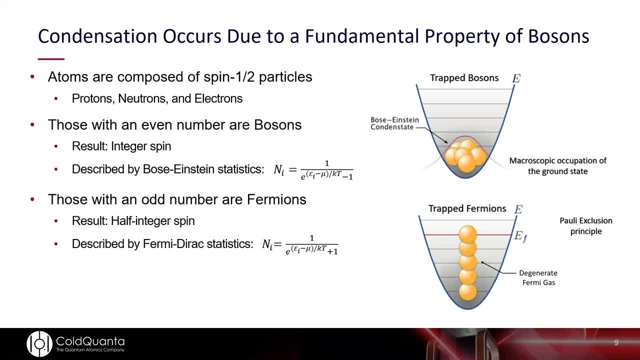 if we were to just look at the two equations, they don't seem particularly different. these, these equations for the particle number to give an energy level, but there is a subtle difference in the sign and the denominator that leads to these difference, these different behaviors. now, when we get back to a range of high temperature, this exponential term in the denominator is much. 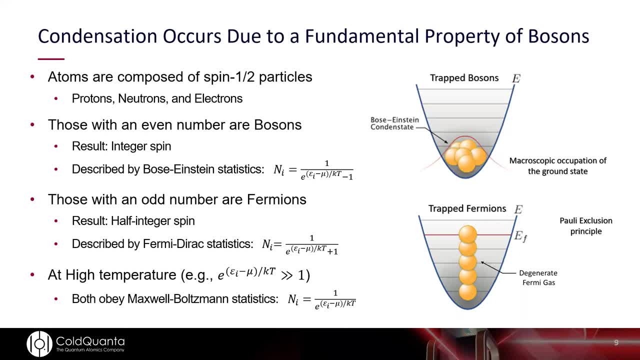 bigger than one, and what that signifies is an absence of quantum behavior. and in this regime of higher energy, higher temperature, we have a system that, again, doesn't necessarily realize either of. these equations are the same, but they are different, and so we have to understand that these two interesting behaviors and instead acts very classically. so this, this transition from 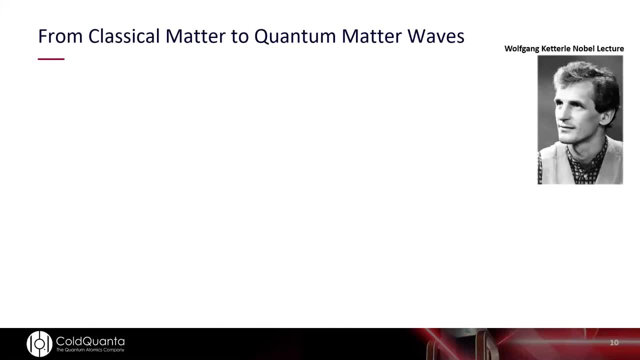 classical to quantum behavior is an important concept and I'd like to borrow the description given by Wolfgang Ketterle during his Nobel lecture that spoke about how classically we can imagine matter waves as billiard, that matter behaves as billiard balls with a mass M. 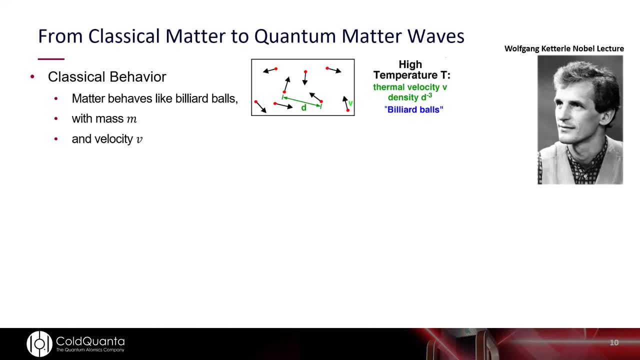 and at high temperature they whiz about with some mean velocity, V, and in a gas, at a certain density they're separated by a distance D, so we can see this cartoon picture here now, when the temperature is significantly lowered, the momentum distribution of these particles, or atoms in this case actually, 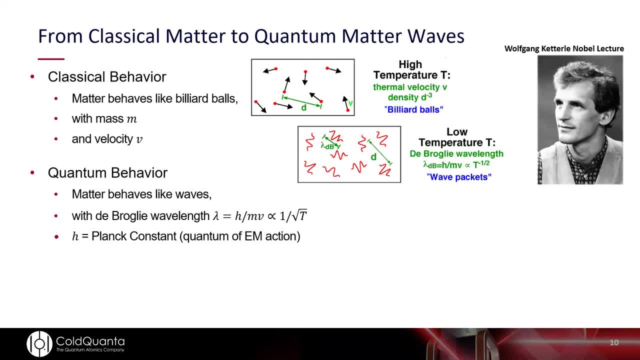 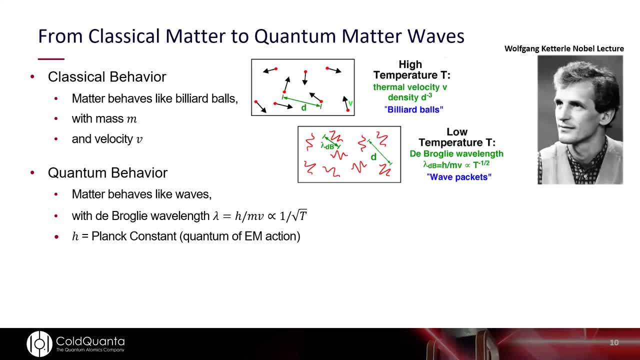 now what that is is effectively Planck's constant divided by the particle momentum, and upon cooling the system even further, it reaches a critical temperature in which the de Broglie wavelength is comparable to the inter particle spacing, and here the wave begins to overlap and coherently begin to be kind of intermingle with other. 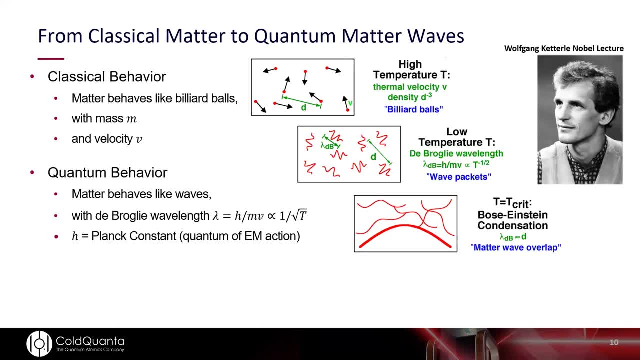 particles, and this is where we get the idea of coherent behavior in the packet of atoms. now, finally, at zero temperature, all the particles collapse to occupy the same state and they behave as a single giant matter wave. and this system embodies particle wave duality very nicely, in which, if we were to take at any moment a look at the system, we would detect particles. 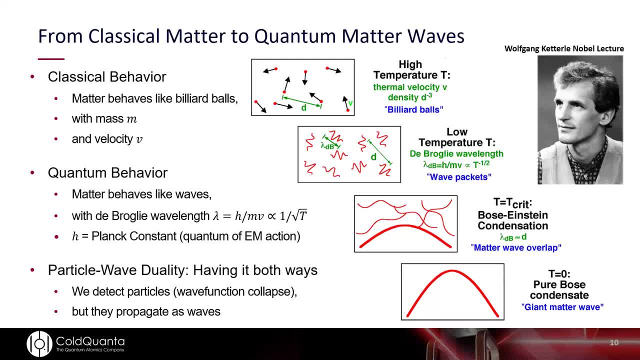 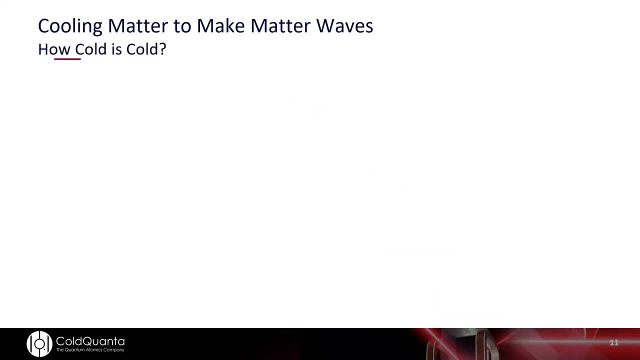 because we collapse their wave function when we look at them, yet up until that point, the behavior that system evolves as if it were a wave. so we've talked about cold, but just how cold is cold? how cold do we need to get these atoms? and it's particularly illuminating to consider a range of temperatures. that's 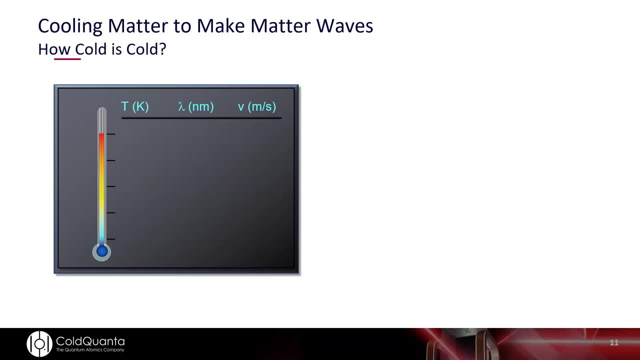 fanned by most experimental BEC systems, and and how that temperature relates to the thermal de Broglie wavelength as well as the, the mean atomic velocity of the sample atoms. So we always begin with a source of atoms near or above room temperature which is roughly 300 degrees Kelvin, and what that corresponds to is a. 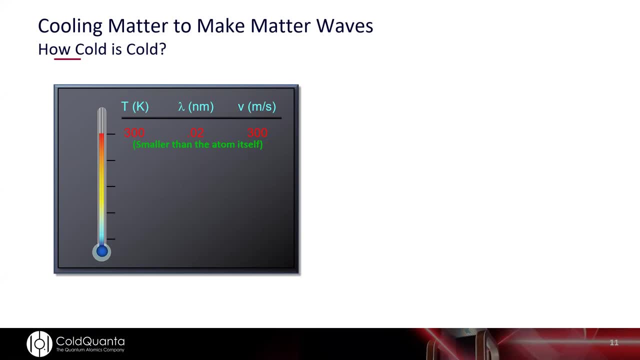 wavelength that's actually smaller than the atom itself, so it behaves very much like a particle. Now, on the other hand, the coldest place in the natural universe is interstellar space or between planets, where there's not much going on and at out there, particles only exist at about 3 Kelvin and at 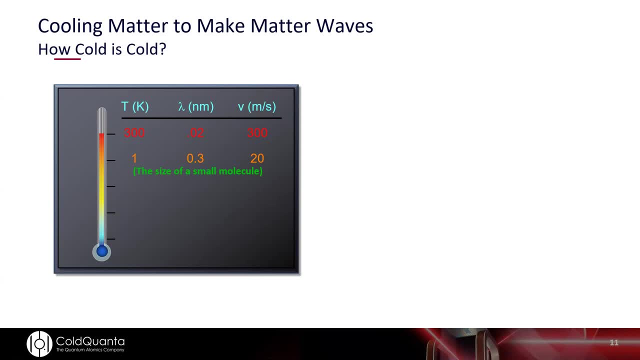 this temperature. the atomic wavelength is on the order of the size of the atom or a small molecule, so still quite particle-like. Now, if we continue with our theoretical analysis, we might be able to see the P-interstellar cool down another factor of 1000 to millikelvin temperatures, which is actually colder than is. 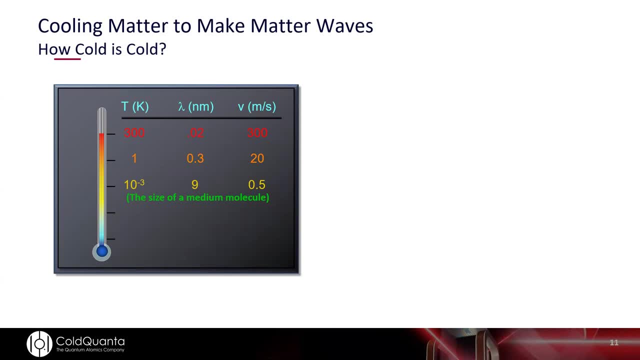 achievable with normal techniques like dilution refrigerators. the wavelength actually increases to about 10 nanometers. So at this point the atoms are quite cold and their speed, interestingly enough, is about that of someone on a leisurely walk. And another factor of 1000 cooler. the atoms reach micro kelvin temperatures. 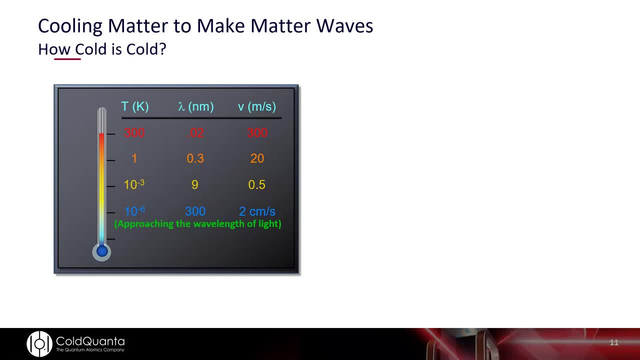 And at this point the wavelength is larger than the atomic radius by about a factor of 1000.. And they literally move at a snail's pace, so a couple centimeters per second, And here some systems that have been produced can actually reach Bose-Einstein. 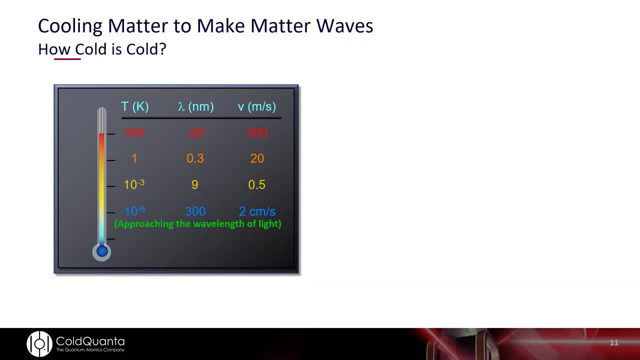 condensate, So roughly a millionth of a degree above absolute zero. But if we were continue to to go down this nano-Kelvin range, we start to see that the wavelength is truly macroscopic Here. 9000 nanometers, that's roughly one tenth the thickness of a human hair. And in this range 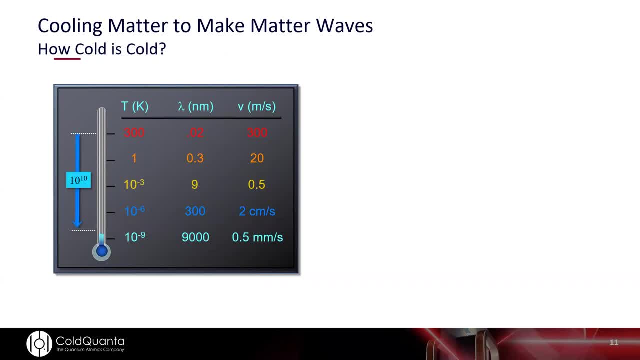 you know, the system can truly be considered a wave. Now, the amazing thing is that if you're looking at this scale, that's 10 orders of magnitude, And it's quite amazing to see that we can control matter across such a wide span, And in order to do so, we need some specialized. 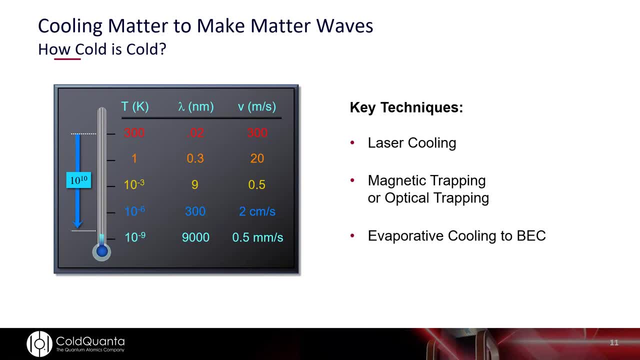 techniques And over the years. these are just a subset of the really important ones, specifically laser cooling, magnetic or optical trapping, as well as evaporative cooling, And these techniques have been so impactful that they've each resulted in three separate Nobel Prizes, with the most recent one two years ago, Art Ashkin and his optical tweezer technique. 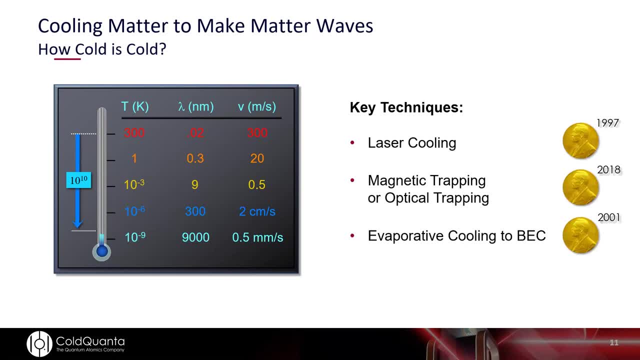 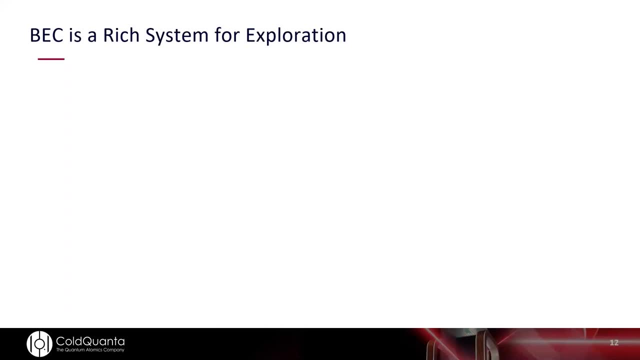 which has been applied to atoms now as well. So now that I've gone a little bit through the temperature range and a little bit more of the subtleties of BEC, I want to get to something useful. So what can we use Bose-Einstein condensate for? After all, it's a very interesting system. 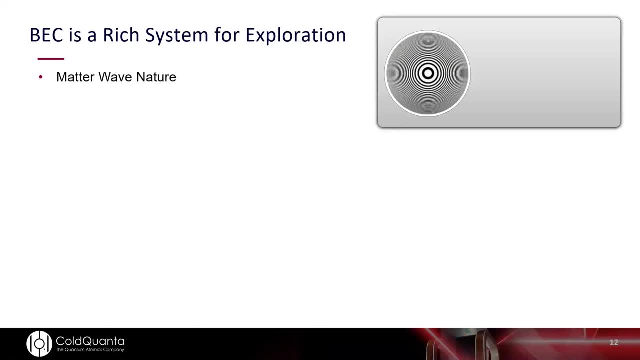 And one of the first features I'd like to point out is its matter wave nature. And so here on the right I'm showing just a cartoon of what the wave function of the atoms might look like as they're expanding. You see, it's kind of a chirped circular fringe where the internal region has a longer. 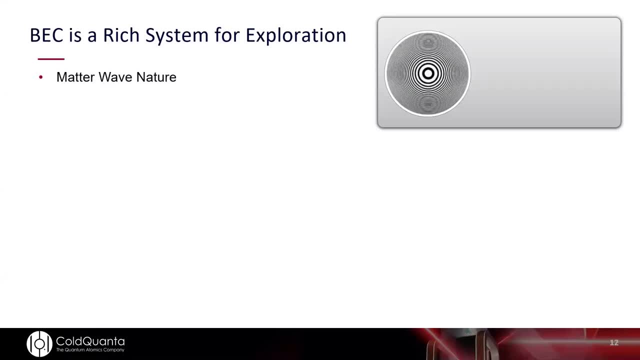 wavelength in the outer region. That's just because the fastest atoms expand further over time. But what's interesting, if you were to have two of these systems and overlap them, you'd actually start to see this interference pattern, And what that is is, in fact, the point. 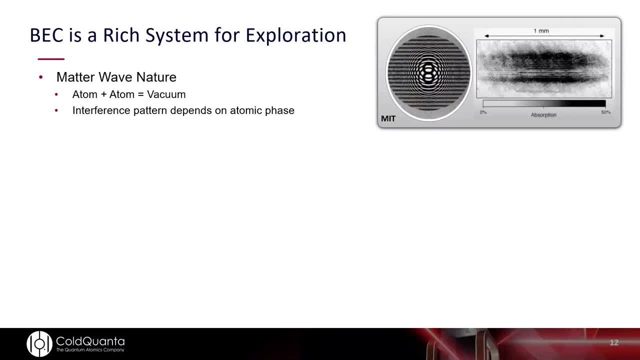 that if you have atoms, they're coherent. they have wave-like nature. when you interfere them, sometimes you actually get the case that atom plus atom equals vacuum And, of course, two atoms somewhere else, And this is really quite a good example of this. 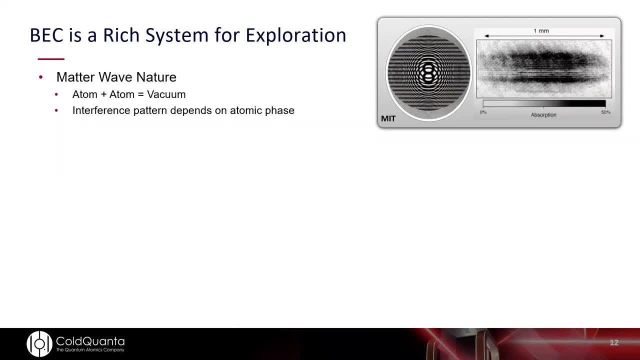 So you get quite a startling image to see. So here on the right we have some old data from MIT where that's the interfering Bose-Einstein condensates that they created, And the important thing here is that now that we can interfere atoms, we can start thinking about making 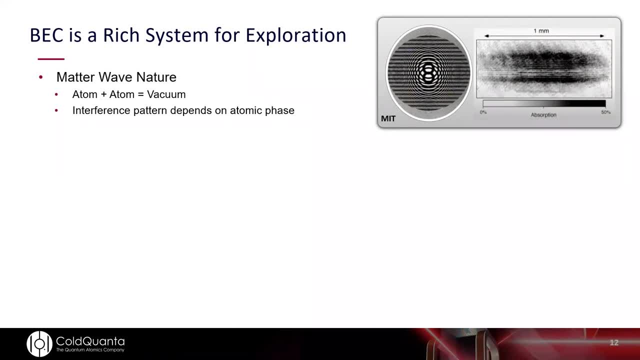 practical devices like interferometers, where the interference pattern depends on phase, much like how an optical interferometer. if you were to change one arm of the interferometer, you'd see the fringes sweep across on the detector. So what that's led to is actually a real rich and deep research topic of atom interferometry. 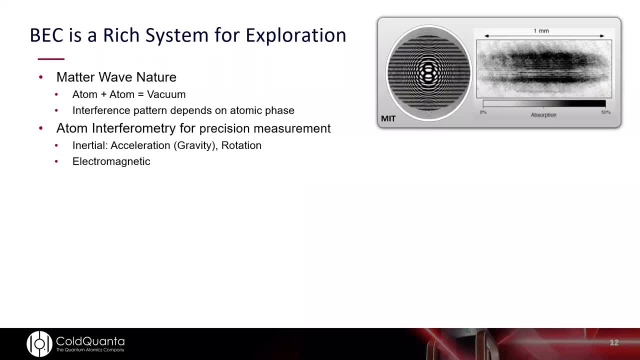 for precision measurement. And one of the other important points about Bose-Einstein condensate of atoms is that they have mass, And because they have mass, they're more sensitive to inertial forces, which more so than photons. you have this amazing sensitivity to inertial forces like 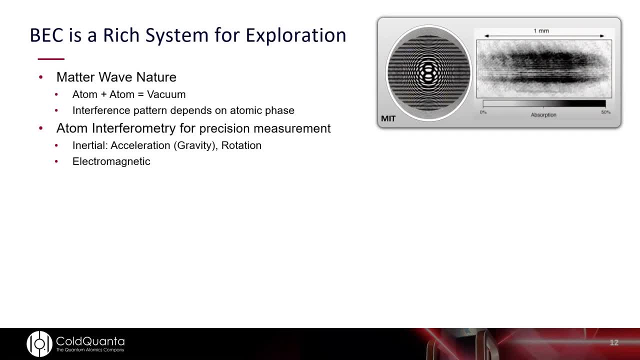 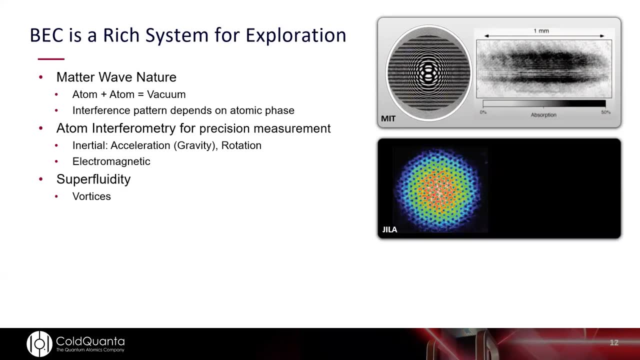 acceleration or gravity or rotation, So we can imagine making accelerometers or gyroscopes of a really exquisite precision. So, beyond being a wave and having mass it, also within the condensate you can observe superfluid behavior, And what that means to say is flowing without resistance. 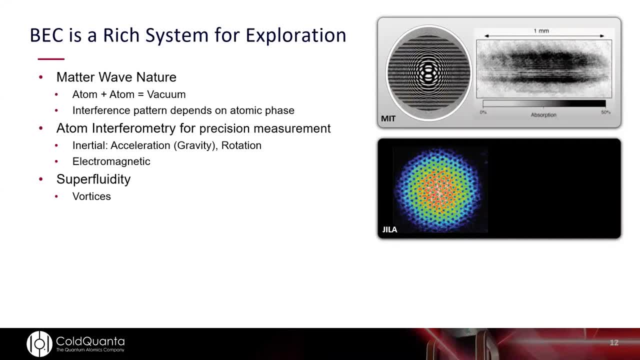 And an example of this behavior is shown in this figure on the right, which is an image of a BEC made in Jilla, And what you see is an array of these holes, And what those holes are are actually an array of vortices where, at each point, each vortex core, you actually have 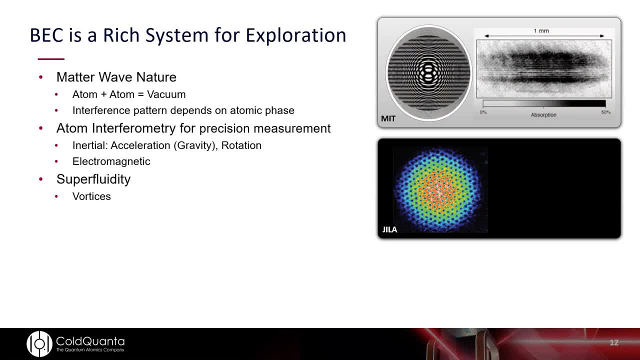 a quantized flow of atoms in a loop whose phase reaches zero to two pi or some integer of two pi, And that density depletion in the middle is in fact due to the fact that the phase has a discontinuity there. So you can see that the phase has a discontinuity in the middle and the phase has a discontinuity there. 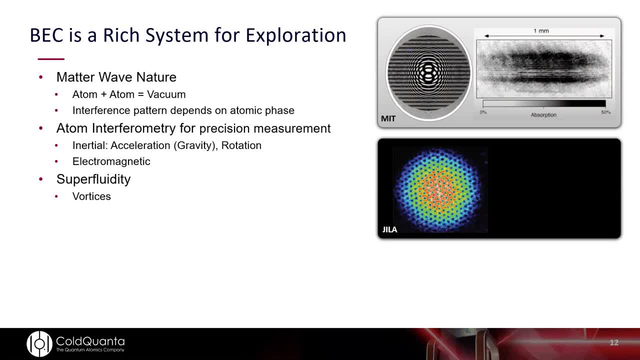 So no atoms can actually be observed occupying that space, And this superfluid behavior actually has been used to recreate some of the physics and the interesting applications of superconducting, Josephson junctions and other quantum interference devices known as SQUIDs. Here's an image from JQI where they make a toroidal trap to hold condensates and then they 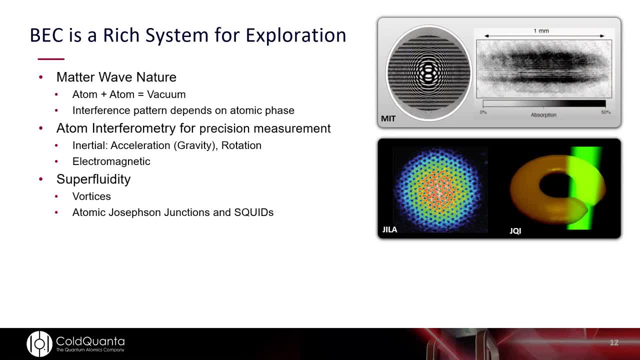 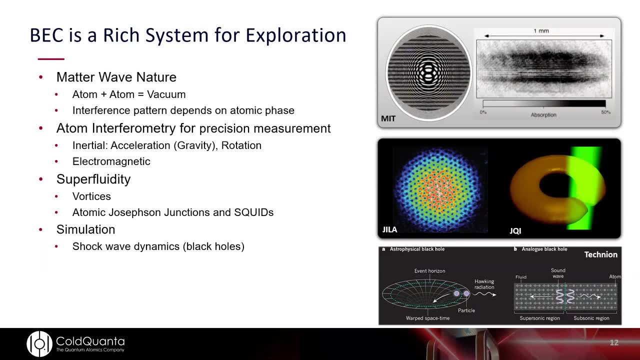 put a barrier in here to act as a weak link for superfluid tunneling. And yet another interesting example, which is getting a little farther from farther afield but actually gives us a really useful control, is the fact that we can use BECs to simulate other systems that are not otherwise controllable. So this figure here shows: 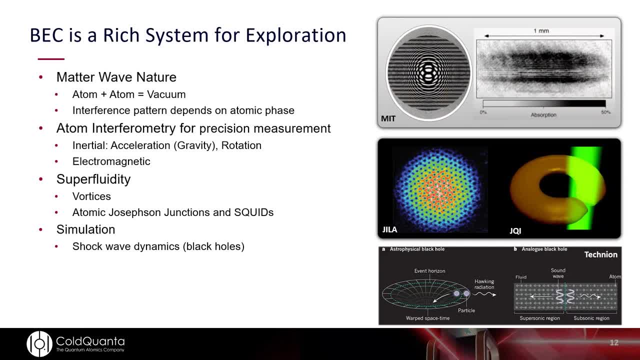 the conceptual link between Hawking radiation near the event horizon of a black hole and the dynamics that are observed in an elongated condensate, where there's a step where atoms can fall down in energy and in fact have sound waves and different sort of shock wave dynamics can be observed. 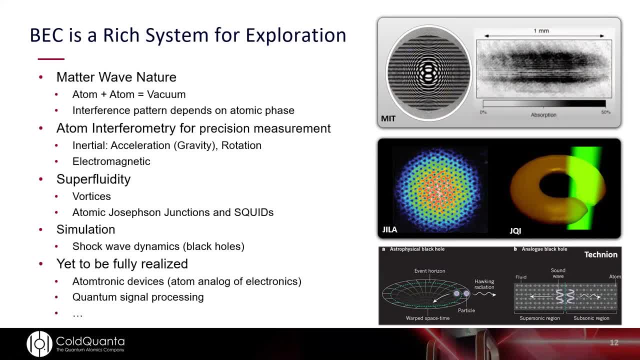 So, you know, these are just a couple of really interesting ones that I could think of at the moment, but there's many more applications to be fully realized. There's this concept of atomtronic devices, which is actually the application of SQUIDs, which is actually the 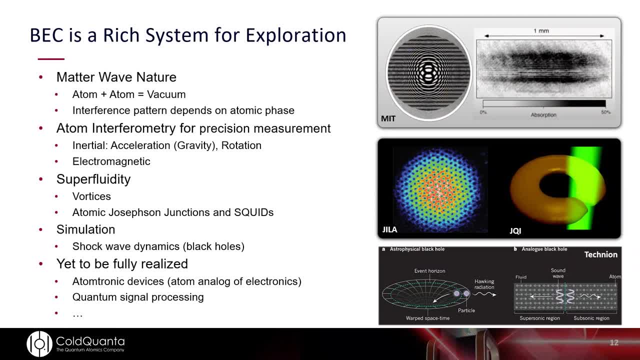 application of SQUIDs, which is actually the application of SQUIDs, which is actually the atomic analog of electronics. We can think about using these atomic systems for quantum signal processing and many more. So I think, without going into an exhaustive list, these are a couple of the 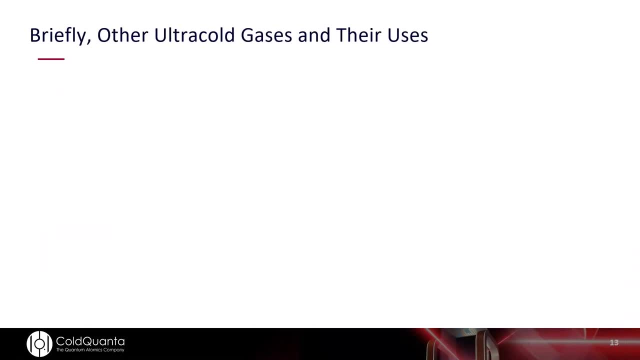 interesting ones I wanted to point out Now. but before I move on to the second portion of this talk, I want to point out that BECs, as I've described them thus far, aren't the only ultra-cold quantum gases to have been created. So 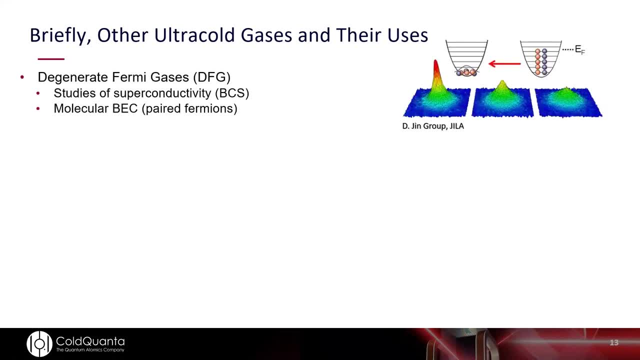 not five years later, researchers at JILA on the CU Boulder campus actually made Fermi degenerate gases. This was the group of Debbie Jin- And this system, even though it's made of fermions, can actually be made to simulate and have other rich dynamics that tell us a lot. 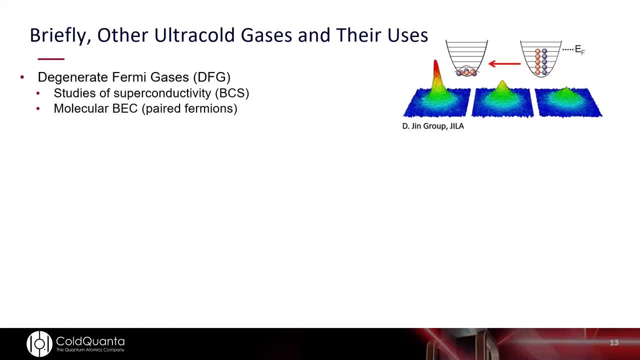 about other systems. So here they actually did studies of superconductivity with Cooper pairing and other systems And they found that the superconductivity of the fermions to reach superfluid behavior, much like Cooper pairs of electrons and superconducting materials, And then also 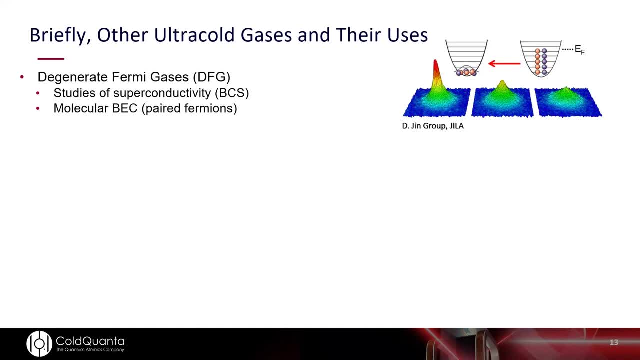 molecular BECs, where you actually take two fermions, form a molecule which now has integer spin and thus behaves according to Bose-Einstein statistics. They actually took fermions and forced them to Bose-condense by making molecules. So in the case of the superconductivity of particles you can actually think about. 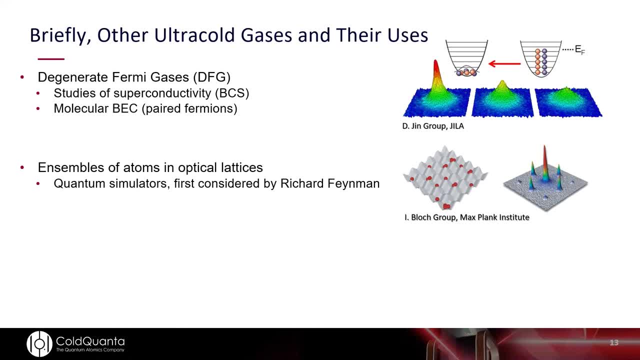 different quantum gases as states of matter that can exist in different topologies or different types of traps. So I talked mostly about these bowl-shaped potentials. but you can also trap atoms in an optical lattice, And what this does is it effectively pins the 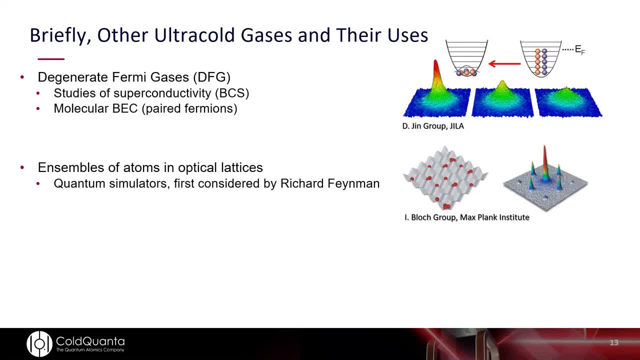 atoms in an ordered grid And we can use these systems as quantum simulators, which first thought of by Richard Feynman, building from the bottom up. And you can actually use these systems to study interesting ordering dynamics, any fermenting ordering, and look at the role of defects or defect-free semiconductor. 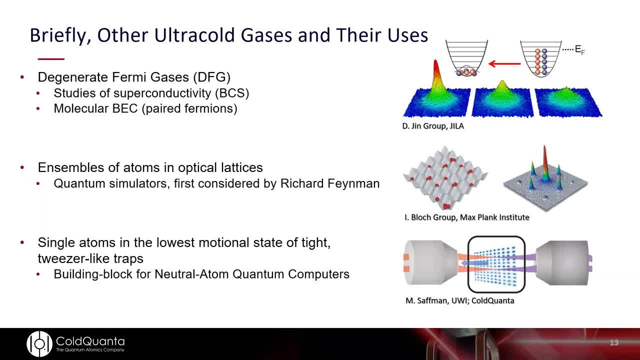 materials. And the last one I'll point out is something near and dear to us at cold-quanto, which is atoms in tweezer-like traps where you have a single atom. So now it's not an ensemble of atoms, we have a single atom and we consider it. 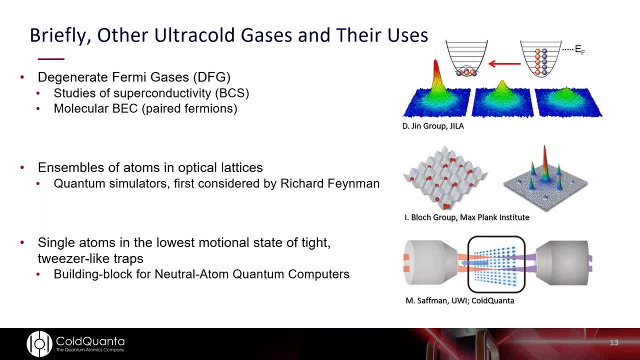 ultra-cold, because it's in this lowest emotional state of the trap And so it behaves somewhat quantum mechanically in that nature, and we use this as a building block for a neutral atom quantum computer. And I don't know when it's to be scheduled, but you should stay tuned. 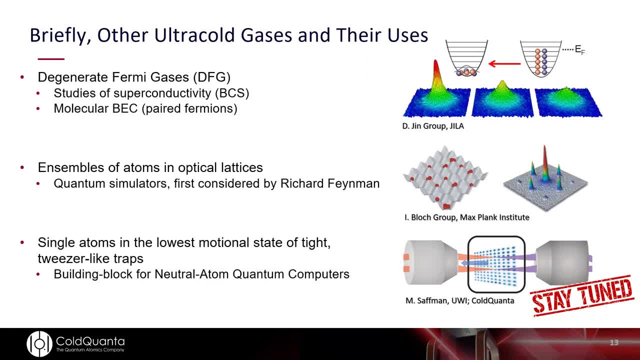 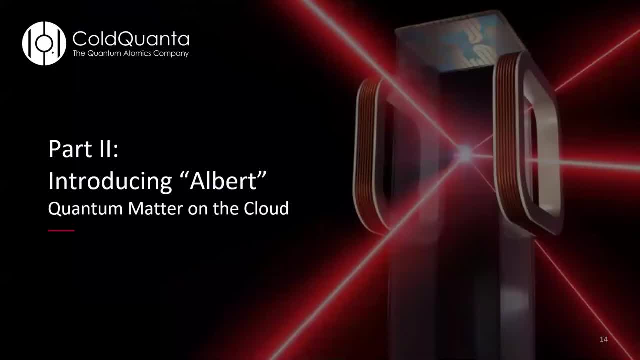 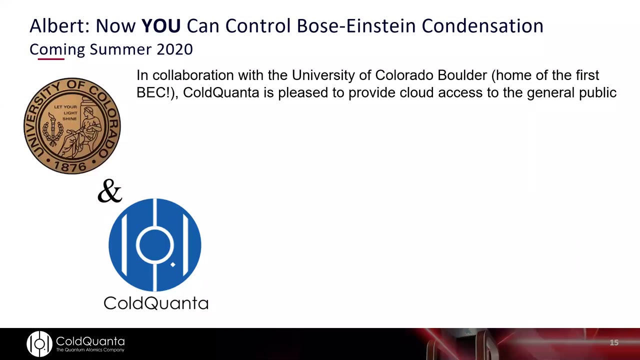 for that. At some point we'll likely have one of our cold-quanto researchers speaking about our quantum computing effort, possibly during this webinar series. Okay, so we're gonna shift gears a little bit and in the second part of the webinar I want to talk about our effort that we call Albert, So what this is and 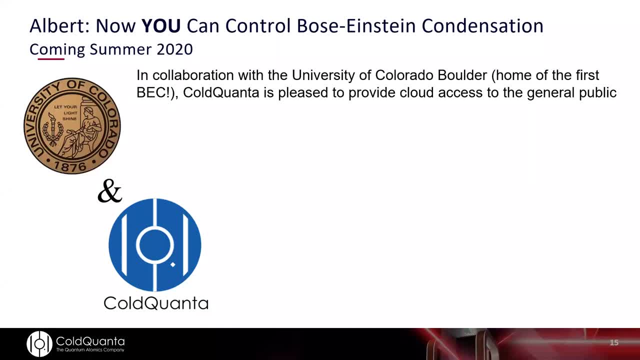 I'm pleased to announce is a collaborative effort between the University of Colorado in Boulder and cold-quanto to provide cloud access to a Bose-Einstein condensate producing system. That is to say, now you, the user, can create, control and experiment with. 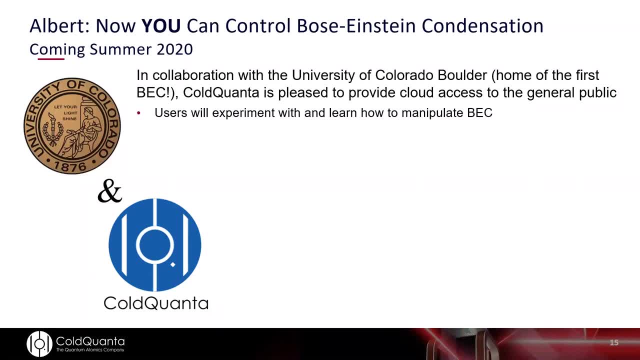 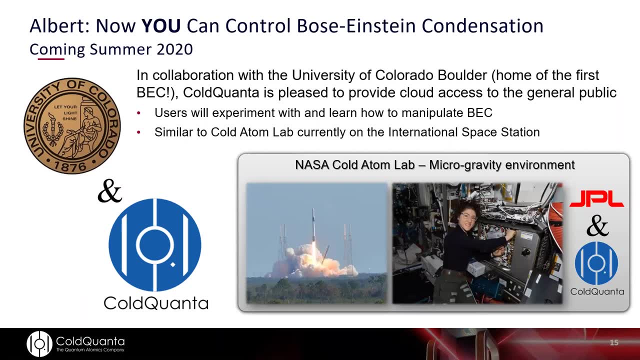 real Bose-Einstein condensates, And it's interesting to point out that this system is actually similar to one that, in collaboration with JPL, cold-quanto provided to put on the International Space Station and is serving for a user facility, a cold-atom lab. The access is unfortunately restricted, but 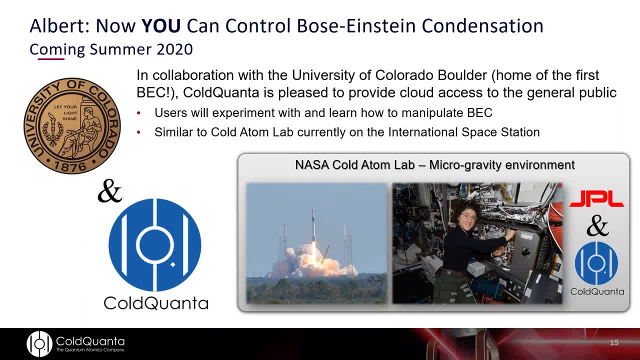 this system gives users down on Earth an ability to remotely control an experiment that looks at fundamental behavior of atoms in a microgravity environment. So while Albert won't give you the microgravity environment, it'll allow you to do more or less the same thing and experiment with Bose-Einstein. 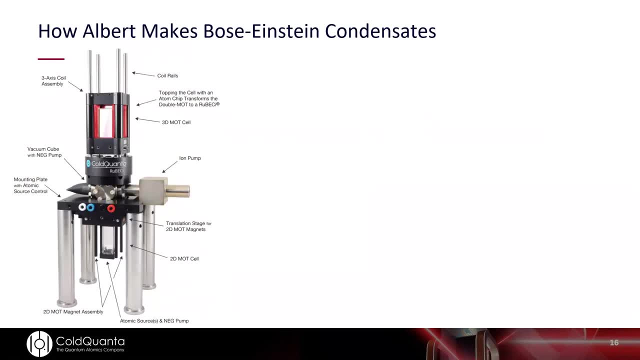 condensates. So let's take a step back to a little bit of technical details. How exactly does Albert create Bose-Einstein condensates? At the left of the screen is a diagram of one of cold-quantum's ultra-high vacuum chambers in which atoms, in this case, 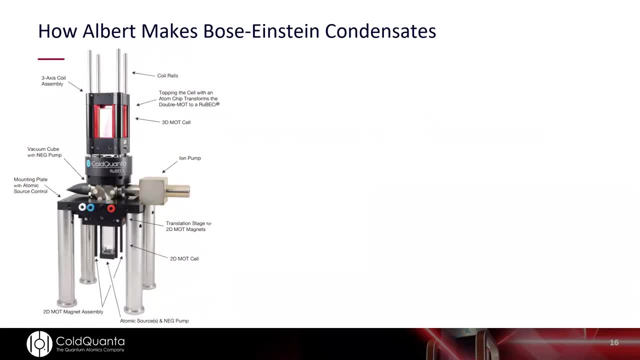 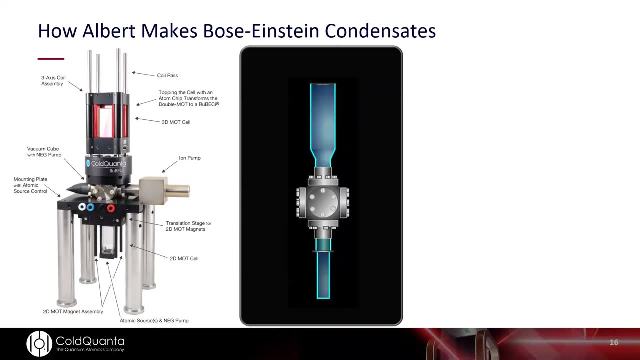 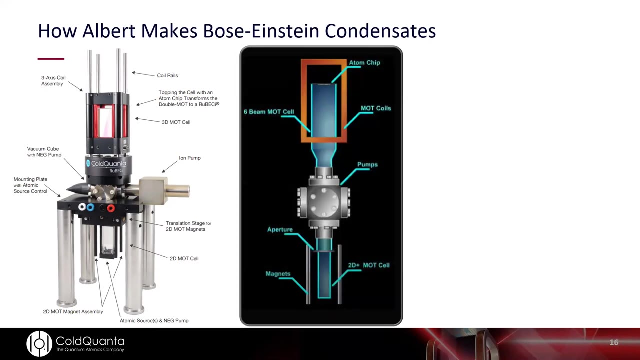 rubidium are isolated from room temperature and pressure. Now, to simplify things a little bit, let's look at this view And around the chamber itself, which has two, an upper and a lower portion, we see these different components: Magnets, vacuum pumps to maintain the 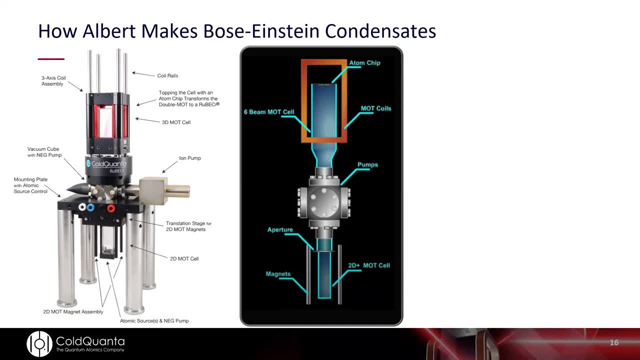 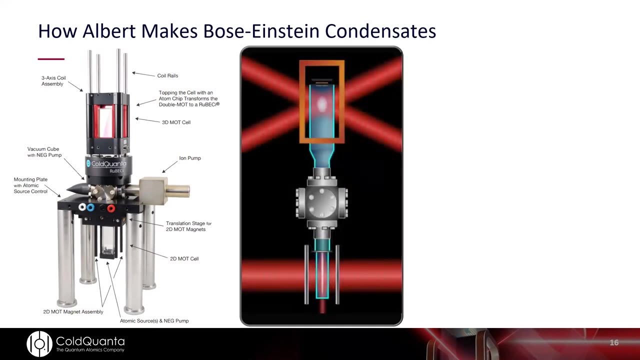 ultra-high vacuum in the chamber. We've got transparent regions where we can put in laser light Mott coils, which are just electromagnetic field coils, and an atom chip up at the top. So in the upper chamber, let's see. so here we had Dana in the last webinar. describe some of the 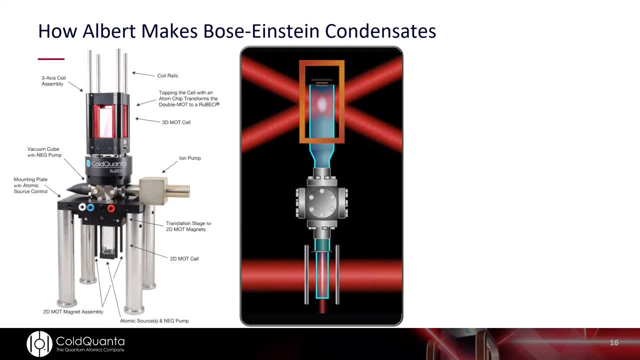 mechanisms that we use to control atoms using laser light and how the Doppler effect works. So I'm not going to go into that, but here I'm showing the two stages of laser cooling that we use in this system. At the lower side we have a 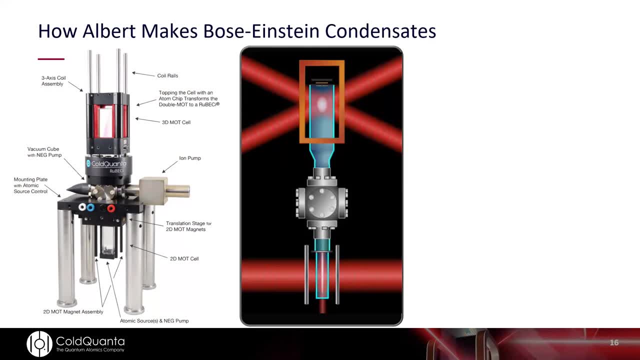 two-dimensional magneto-optical trap. This takes atoms that are heated out of the source, cools them and then shoots them up in a jet to the upper chamber. We do more laser cooling and in the Upper Mott the temperature. 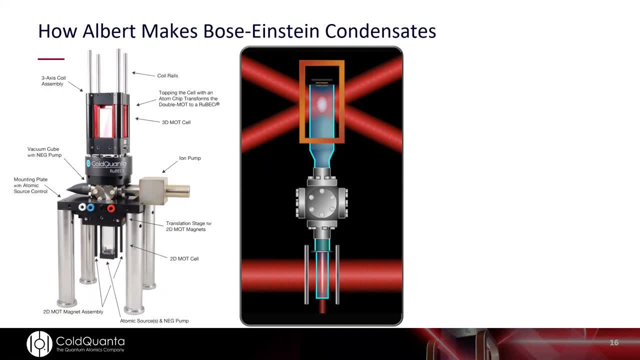 of these atoms is already reduced to less than 1 millikelvin, And after a few subtle changes in the frequency of the laser light and magnetic fields, the atoms reach tens of microkelvin, So tens of millionths of a degree above absolute zero. Now if we zoom in a bit at this, 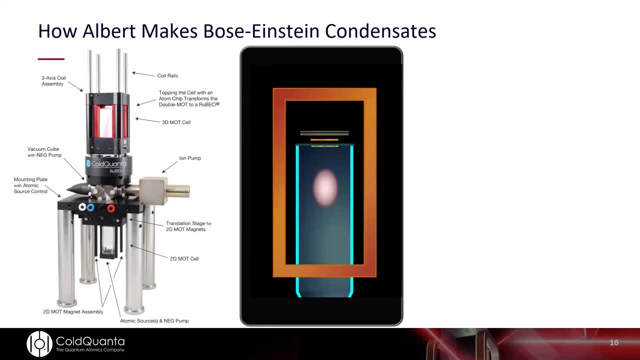 point, the light is extinguished and we capture the atoms in a bowl-shaped magnetic trap. And to cool the atoms to form a condensate, the atoms have to be tightly confined or more tightly confined such that evaporative cooling is efficient. 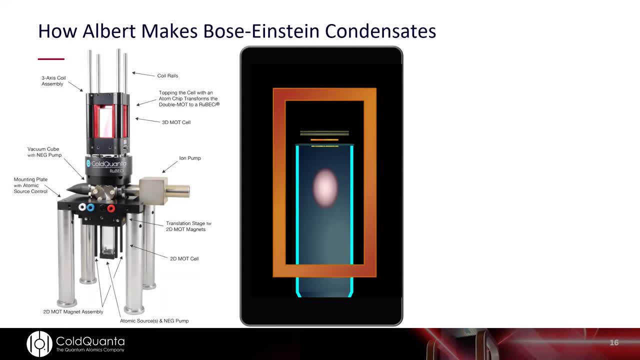 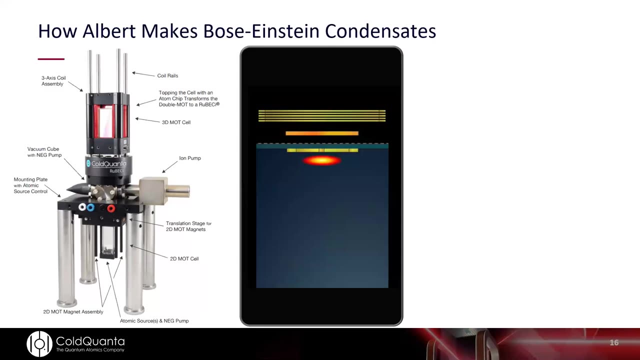 And what this requires is a tighter trap where atoms can undergo a higher ratio of good collisions that aid in the cooling process to bad collisions, which either heat the atoms or kick them out of the trap. Now, there are many ways to achieve this, but in our case, we transfer the atoms into an atom chip magnetic trap. 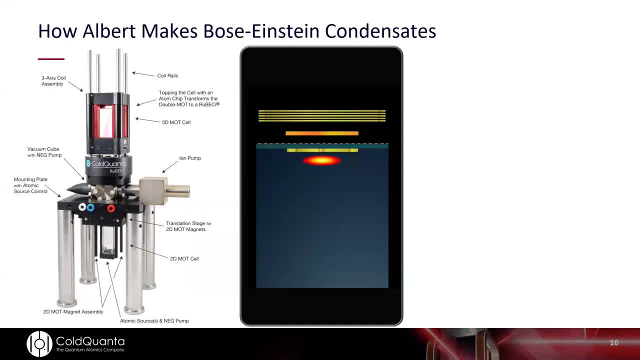 The atom chip at the top of the vacuum chamber includes thin metallic traces through which we flow electric currents to create this tighter trap, And it's much tighter than we can otherwise make with large coils outside of the vacuum chamber. Now, once atoms are in this chip trap, we begin evaporative cooling. 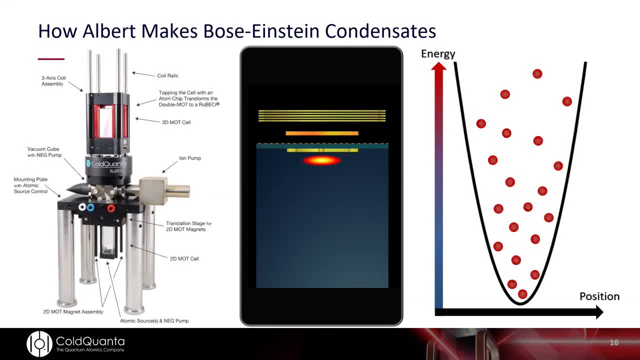 And to illustrate how this works, we can imagine atoms in this parabolic potential, where they're distributed according to their energy and they're whizzing around and they're colliding, And once the atoms are in this trap, we apply what's called an RF knife. 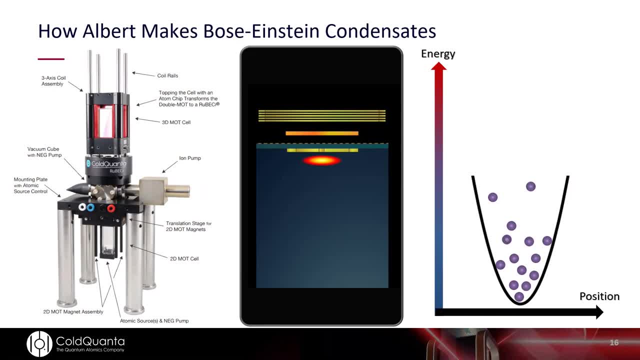 And what this does is it selectively removes atoms of higher energy than the average energy of the particles in the trap, And what that does is it allows the removal of higher energy. And what that does is it allows the removal of higher energy than the average energy of the particles in the trap. 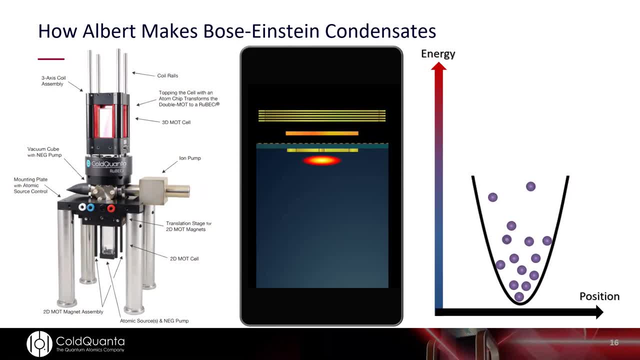 It allows the remaining atoms to redistribute their energy and become, on average, colder. Now we do this multiple times where the atoms collide, come to equilibrium and we remove more through another addition of an RF knife And you are repeating this process until we achieve the temperature that we want, in this case forming a Bose-Einstein condensate. 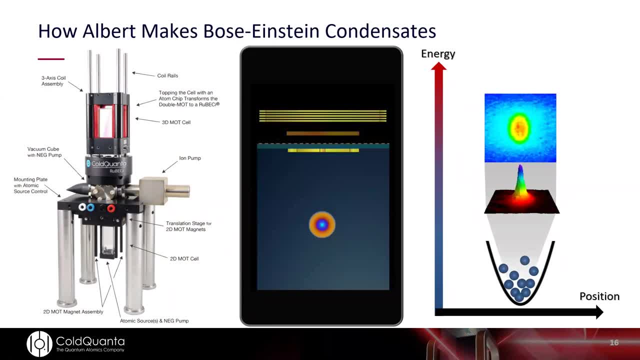 After the condensate is created, we like to observe it. So what we do is we release the atoms from that magnetic trap and then we take an image by shining resonant light on the atoms, and the atoms, according to their density, absorb the photons and cast a shadow on the imaging device in the camera. 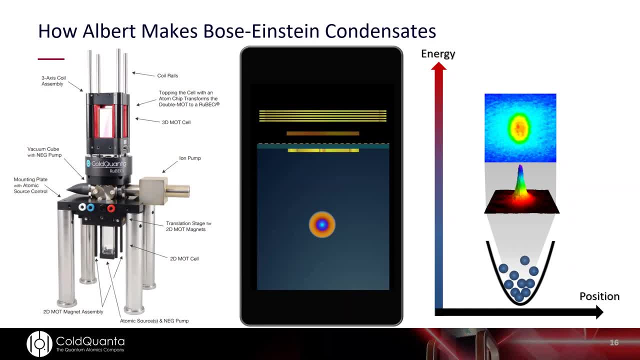 And what I'm showing here on the right is two different types of images that one might see. The lower one, this three-dimensional distribution of density, with the high peak in the middle signifying the condensate, or, most typically, we just see this two-dimensional image that we color code. 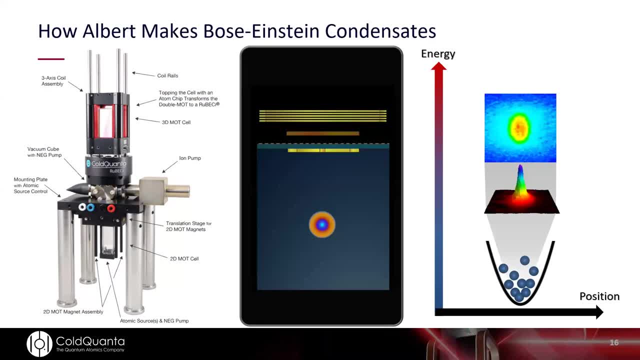 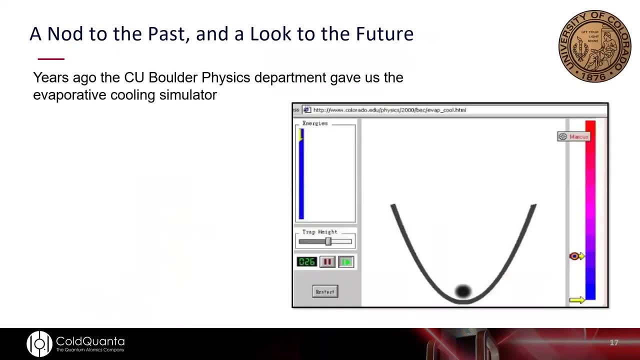 And you can tell a lot from these types of images and this is typically the tool that researchers will use to characterize BEC. And maybe some of you recall, years ago, after the first BECs were created, the physics department at CU Boulder created these little applets for folks online through the internet to experiment with evaporative cooling. 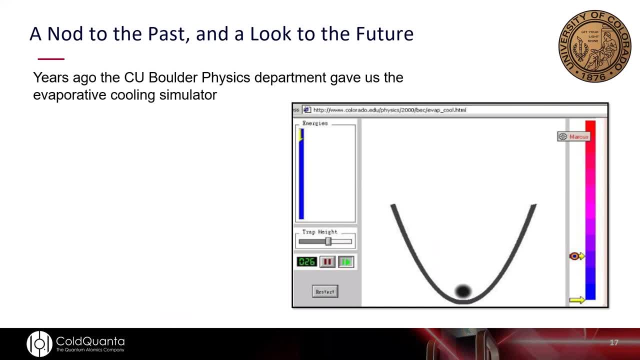 In this case it was just a simulator where you could control the trap height, in a way controlling the RF knife that I was just talking about, And they even challenged their users, or at least they challenged each other, to see who can figure it out. 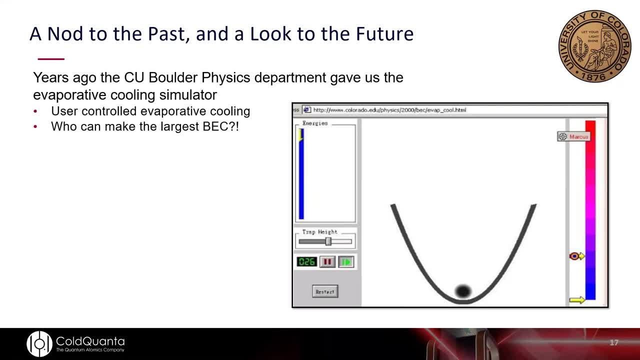 And they even challenged their users, or at least they challenged each other to see who can figure it out. And they even challenged their users, or at least they challenged each other to see who can figure it out. And that is to say: well, with Albert you can do the same thing, only this time you're doing it with real atoms. 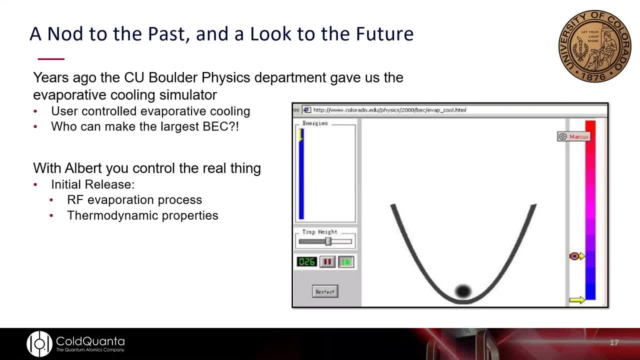 You're learning about the real techniques that go into forming Bose-Einstein condensate, And more so than that, you can start to learn more and really explore these more useful fundamental properties, like the thermodynamic properties of an ultra-cold gas. 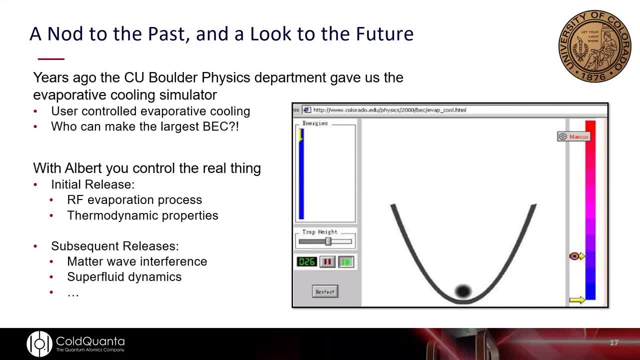 So what I've talked about so far is what we imagine will release first, but in subsequent releases we fully expect to give the user control over more novel concepts like matter wave interference I just spoke about, or superfluidity, And now we can view this kind of as an evolving system. 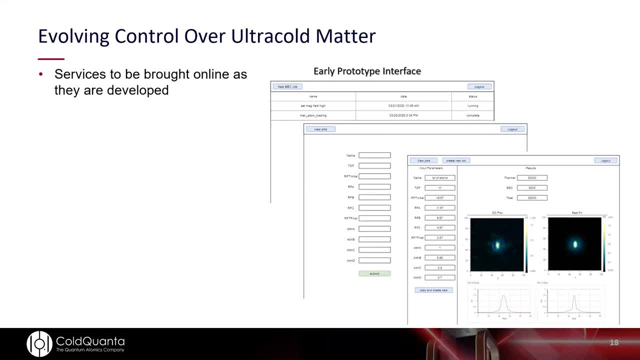 We can view Albert to be growing up over time, And what we want to do is have users be able to store and retrieve past experiments, compete with others if they wish or develop theories of their own, And here you can see some images from an early prototype interface which shows different 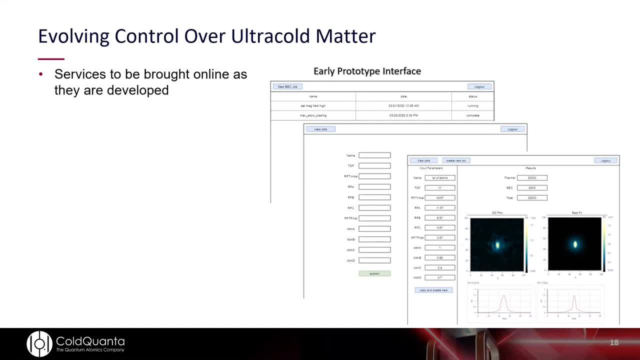 types of input parameters. One might have a job selection screen, a screen controlling all the different variable inputs, as well as one to show you the results of your experiment. And in addition to just having control, we want to help you by providing tutorials to 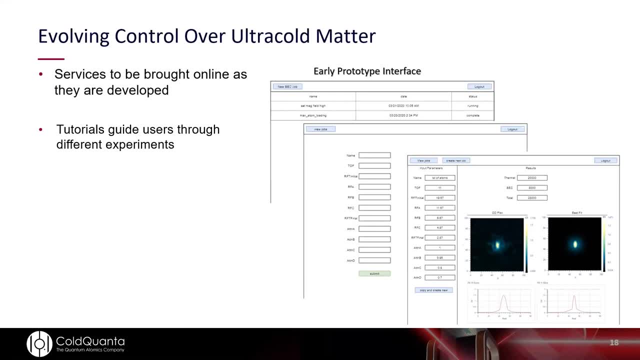 guide the users through different types of experiments. So there will be preset experiments with a tutorial to teach you not only about the original experiments that found these different types of behavior, but allow you to then take that template and then create your new experiments that go beyond what's been done so far. 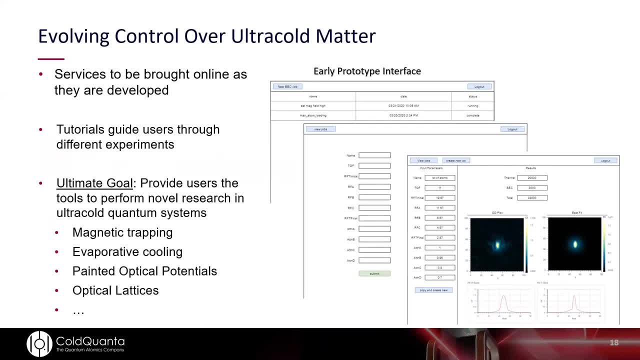 And the ultimate goal is to give users the tools to really perform novel research in a way that so far has been limited. by access to these types of machines, You typically have to have be either part of a lab or be real good friends with someone. 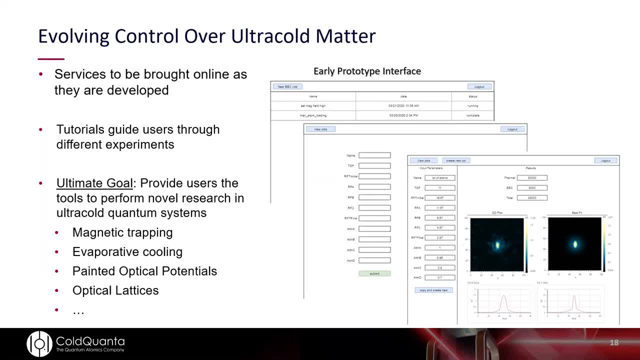 in a lab who will let you go in and actually toy with their large, complicated apparatus, And in this way you don't have to worry about upkeep, But instead you can focus on the results. So that's the ultimate goal. 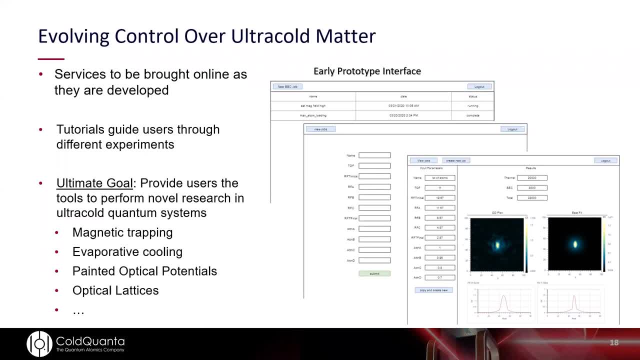 And the last thing I want to talk about is the research that actually interests you, And so here I've just listed a couple different types of components and techniques that we'll implement in the system in the coming days and months, And, because everything is connected through mobile devices these days, we'll even make 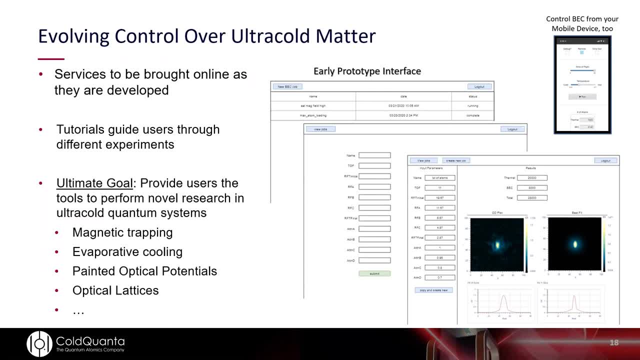 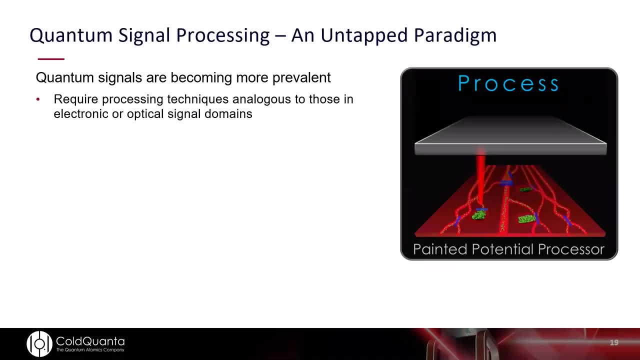 sure that on a plane ride or somewhere in an Uber, you can start working with these too and control it from your phone or tablet. Now, there's a lot of things you can do with this type of system And I'm not going to go through all of them, but we had some nice webinars discussion from 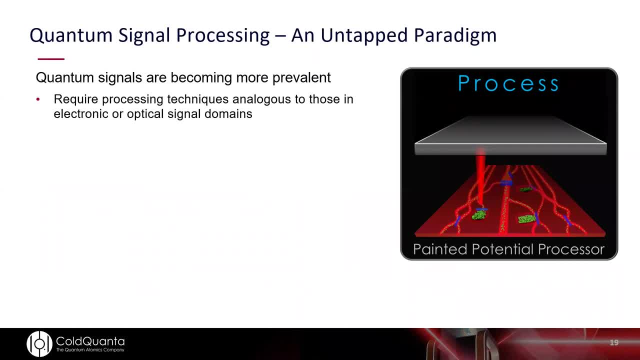 Bo and Dana and they talked about some of Colquana's primary interests, And the first one is actually quantum signal processing, And we find that our world is continuing to develop quantum technologies and quantum signals right, So we need to have some sort of tool box for signal processing. 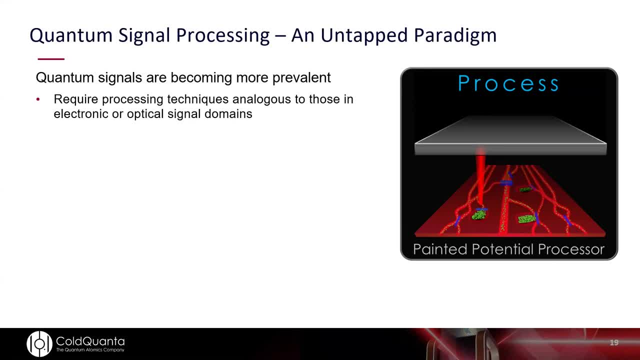 And, much like the role of electronics and photonics, we're going to do this with atoms. In this case, the atoms and the photons will be the carriers of the quantum information, And in order for them to behave coherently, we need to have some sort of way to produce. 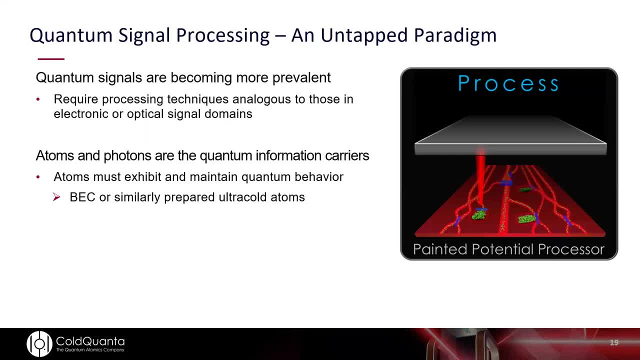 and maintain that wave-like nature that carries this quantum information, And so a BEC or similarly prepared ultra-cold atoms is where we're going to start. Next, you require some sort of circuitry that actually performs the tasks that you want. 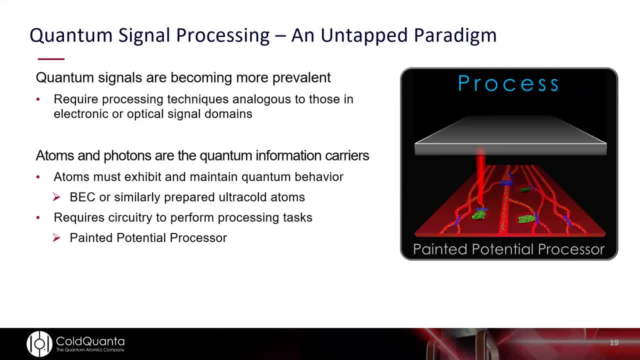 these processing tasks And we have shown in this cartoon on the right an idea of a painted potential optical atomic processor that allows us to do some really interesting quantum information processing techniques And thankfully, because of that, we're going to be able to do some really interesting quantum. 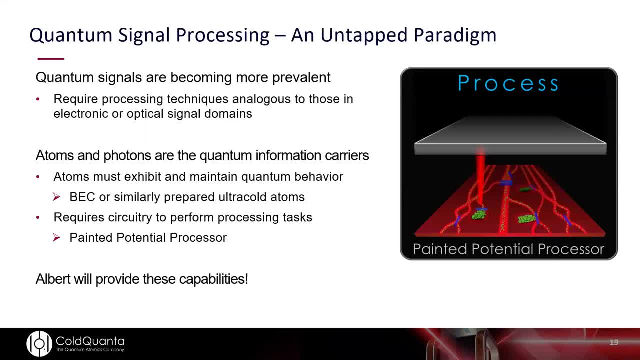 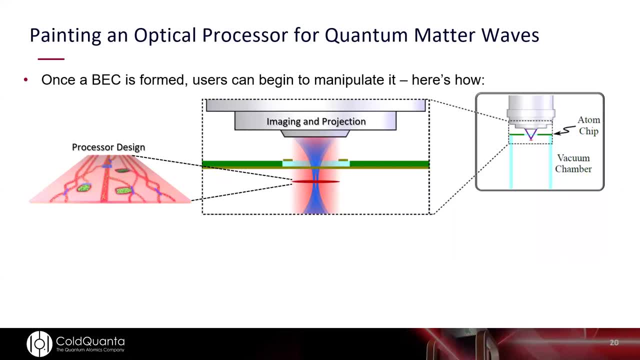 information processing techniques And thankfully, because of that, we're going to be able to do some really interesting quantum information processing techniques And thankfully, because of that, we're going to be able to do some really interesting quantum information processing techniques. Now, of course, we want you to also have these techniques to play with. 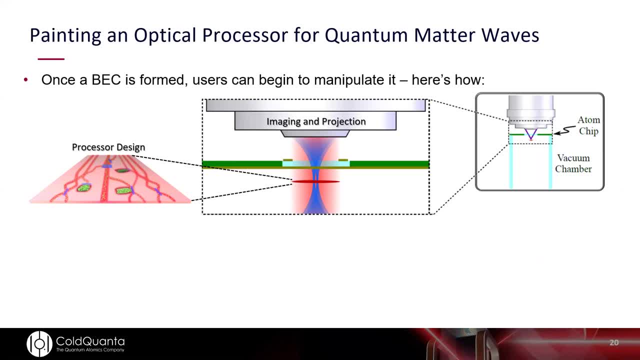 Albert is going to enjoy these capabilities as well. So, digging a little bit deeper, how exactly does a painted optical processor work, especially for quantum matter waves? And I like to just kind of schematically show it in a couple of images. So on the left, after we've made a BEC and we've preconceived this processor design, 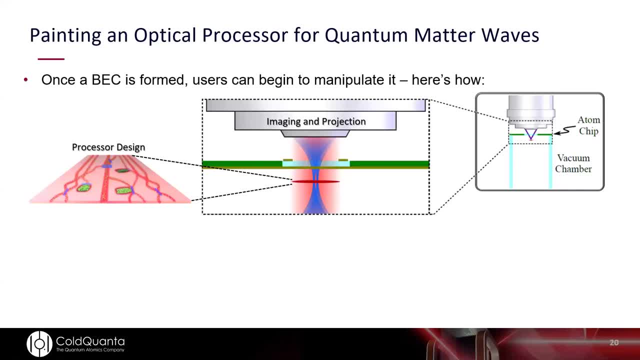 where we've got red light attraction, black light attracting atoms, blue light repelling atoms, as Dana talked about in the last webinar series. We project this onto the atoms, whether it be in a magnetic chip trap or some other sort of trap. 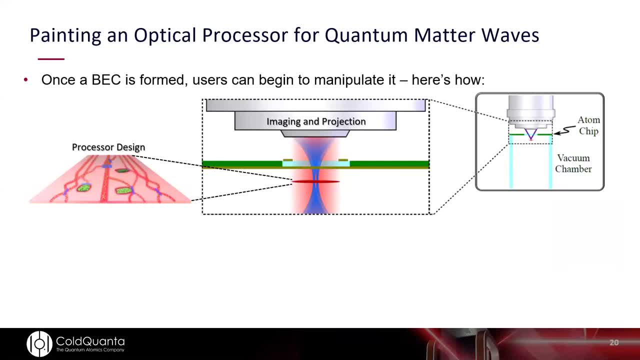 And here I've shown a diagram where there's some microscope objective that lives outside the vacuum chamber and some other optics that we use to project this optical processor design down onto the atoms, And we can initialize this circuit and then allow the dynamics to proceed, after which. 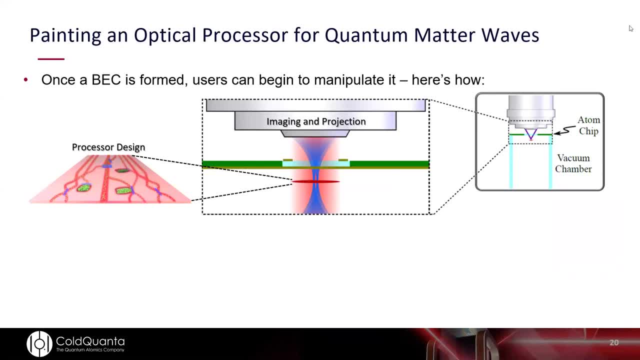 point we can image and look at the results. And just to again tie this sort of system back into what I showed in earlier slides, in this case we've got an atom chip with a window in it so we can see the atoms up close. 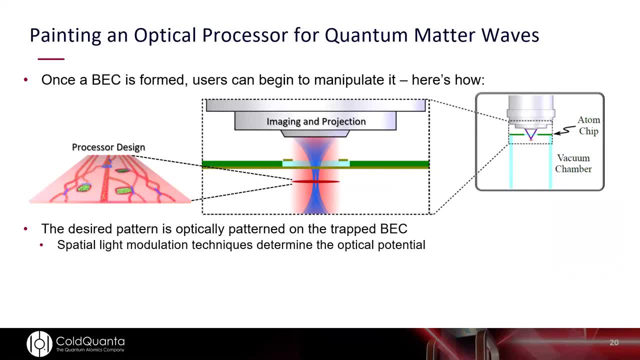 and project these potentials down on them. And now the interesting thing is that, because this process is so complex, it's so complex that we don't have enough time to actually do anything about it. So, even though this optical processor is made using spatial light techniques, you can actually 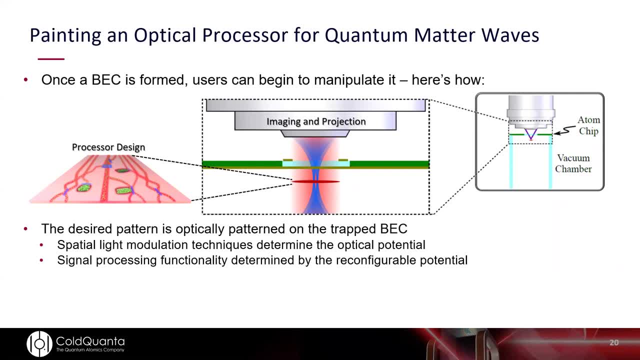 think about changing the functionality over time, evolving it, improving it, because it really is a reconfigurable potential. So, even though we're making something to do a particular function, it's made of atoms and light and it doesn't have to take a solid form like a semiconductor chip. 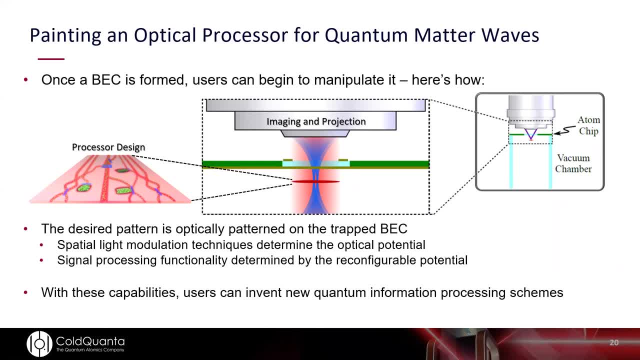 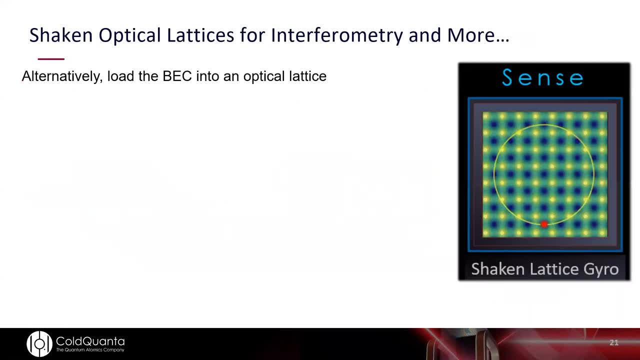 And so, with these capabilities built into Albert, we really have to think about how to do this, and we really hope users can invent new quantum information processing schemes and show us things that even we haven't thought of yet. Now the next one. the topic that Dana spoke on a little bit is the concept of what you 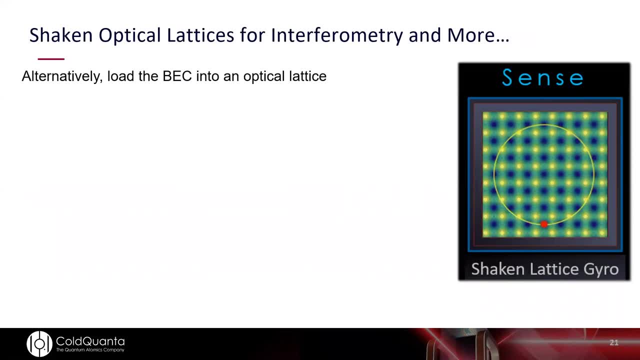 can do with atoms in an optical lattice, And so here, starting with the BEC, we put it in an optical lattice which is effectively just three pairs of counterpropagating laser light, controlled in a specific manner, can start to get at some of these other ultra cold quantum gases that I briefly 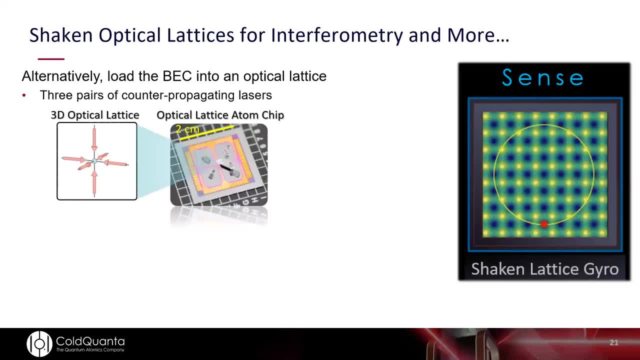 mentioned earlier And, just as an aside, ColdQuant has done some interesting work in this in the past. Here we had a customer who was interested in having an optical lattice on one of our atom chips. So you can see some micro optics bonded to one of these chips with a window in it And, importantly for the future, of 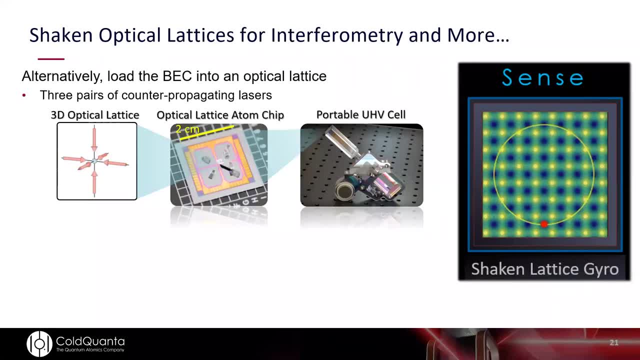 this type of system, which is actually really useful for things like inertial sensing, because this egg crate, like potential, confines atoms with forces of tens to hundreds of G's. you could imagine putting this chip on one of ColdQuant's portable UHV cells, and now you've got a device that can be taken. 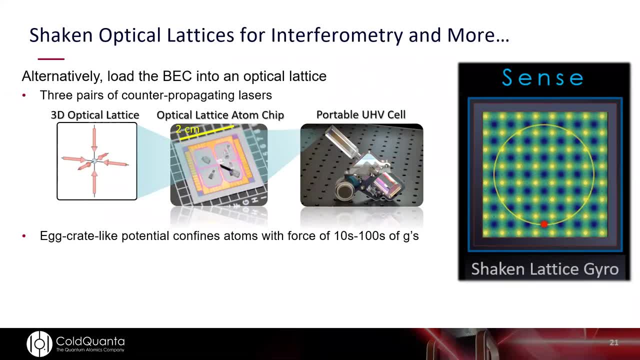 out of the lab and used as an inertial measurement unit on some moving platform. And what we imagine here is that this chip can be used as an inertial measurement unit on some moving platform. And what we imagine here is that this laser light that we're confining the atoms with in the optical 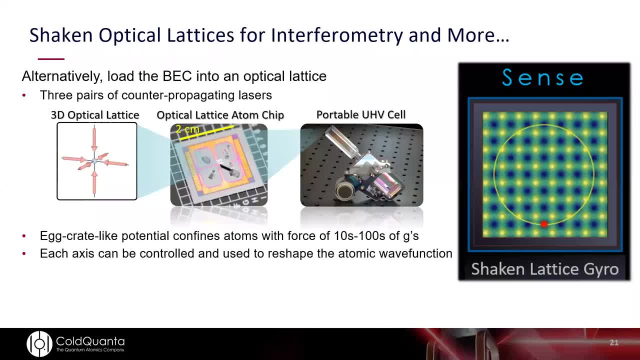 lattice can actually be controlled in a way that can reshape the atomic wave function, And whether that be for what's shown on the right here, kind of as a cartoon where you're controlling atoms moving around in a circular trajectory to make an optical lattice gyroscope, or if it's some sort of more complex wave. 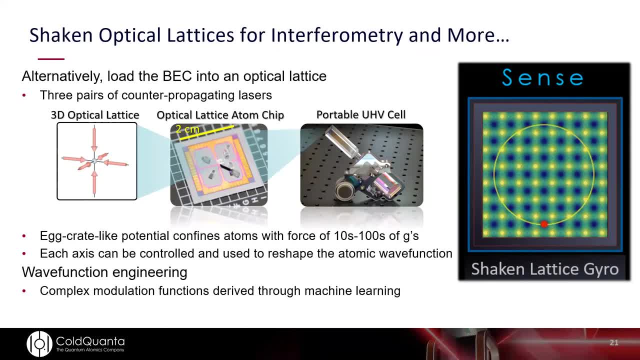 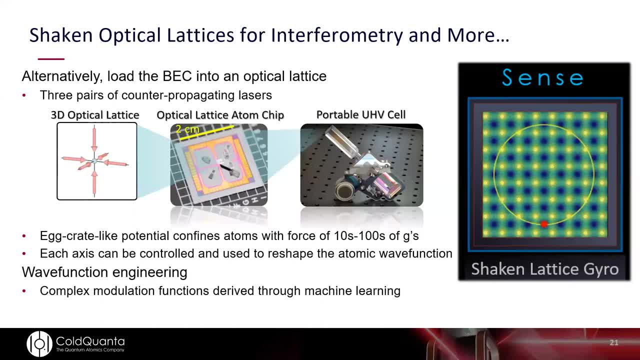 think maybe we've arrived through some Now. we can get it the concept of quantum machine learning, and that's a deep coming, And we can get it the concept of quantum machine learning, and that's a deep topic that hopefully we can get to in a future webinar series. But it's it's. 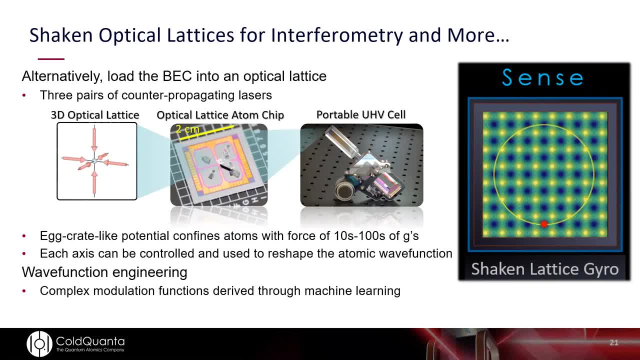 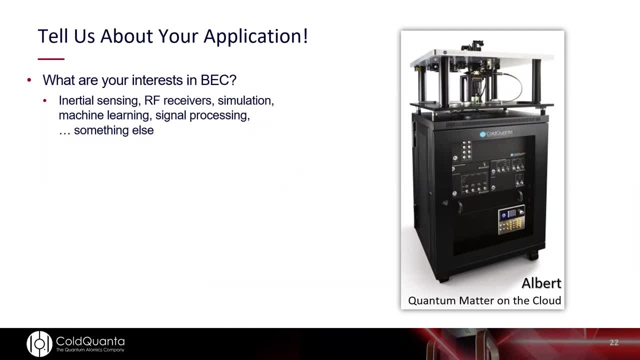 really interesting and this type of technique with modulated lattices is a really interesting and this type of going be available on Albert as well. So I've told you a lot of things today about what be able to be available on Albert as well. So I've told you a lot of things. 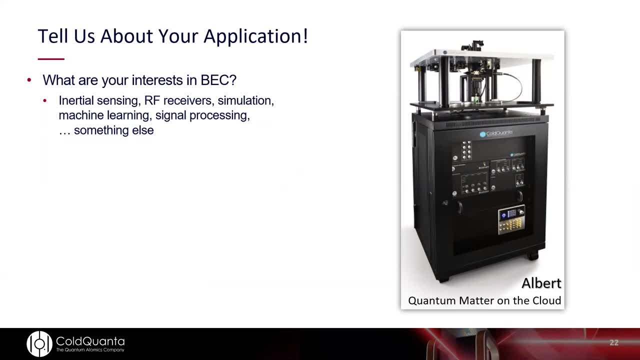 stol cocác. it is how Albert can let you chrome and fiction and electronic data, that opportunity. So I want to thank you, control Bose-Einstein condensation and do interesting ultra-cold atom research. But what are your interests? Inertial sensing. 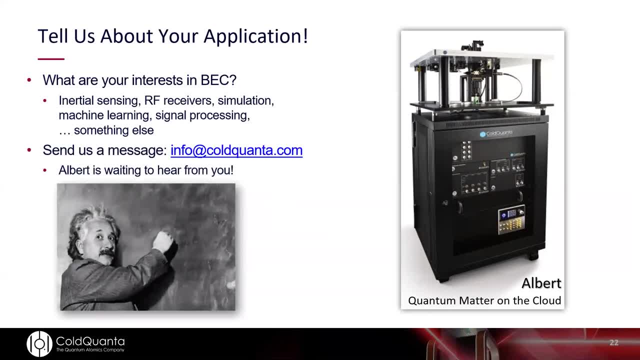 receivers, simulation signal processing, maybe it's something else. So I invite you to actually send us a message at info at coldquantacom, the same email address that was mentioned earlier, Because we at Cold Quanta, as well as Albert, are waiting to hear what you want to do with this type of system and 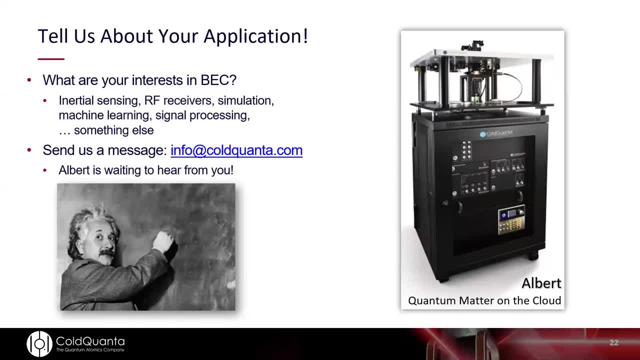 if we can, we'll try to accommodate your interests. And here, whether you think of Albert Einstein or not, Albert really is one of Cold Quanta's or eventually will be one of Cold Quanta's machines We're starting with in collaboration with CU Boulder, so we're kind of building up to having multiple of these sorts of 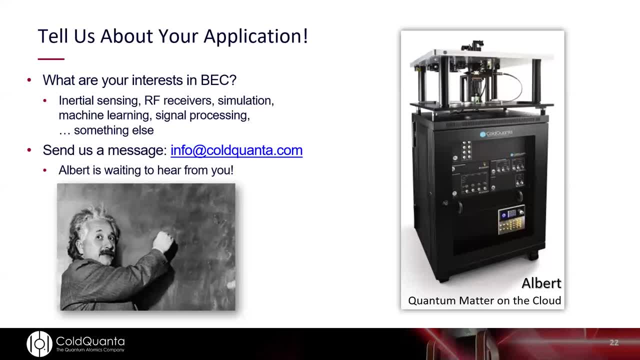 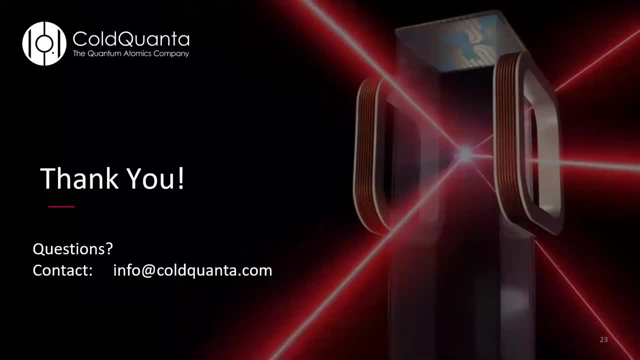 Albert-type machines built at Cold Quanta, Where we can put quantum matter on the cloud for folks like yourself to use and experiment with. So, with that, I think that's all I've got for today, and I really appreciate you attending today's webinar and 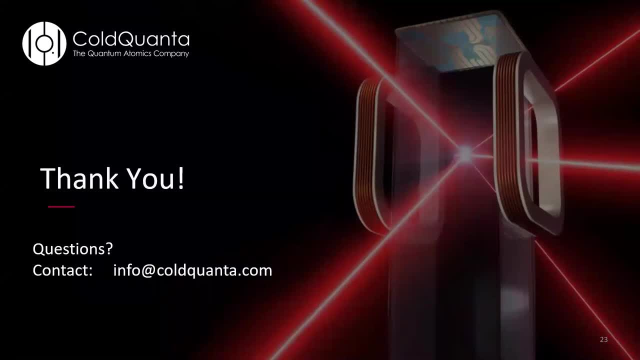 at this point I'm more than happy to answer some of the questions that you may have been sending in through the Q&A dialogue box. Thanks so much, Seth. So I have a couple of questions here for you. Are the wires making the trap not in the way of? 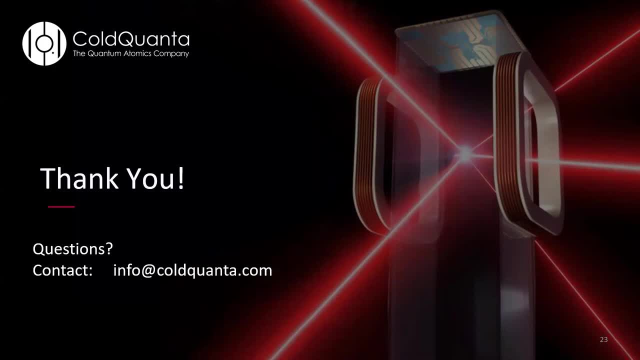 the optical lattice window and why shine the potential painting laser from the top. Okay, those are both good questions. So we actually have. we actually have chip wire designs that allow us to not have the wires in the way. I won't go into the details. 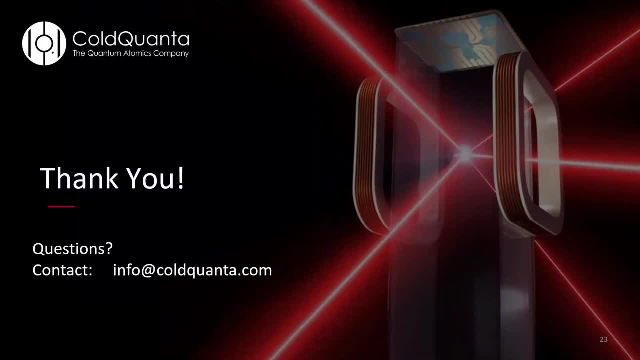 but there's certain configurations where you can have the atoms trapped not directly beneath the wire and in that way there's clear aperture in the window and that allows you to access the atoms through the chip optically, and then it does not have to be from the top, It could be in some other. 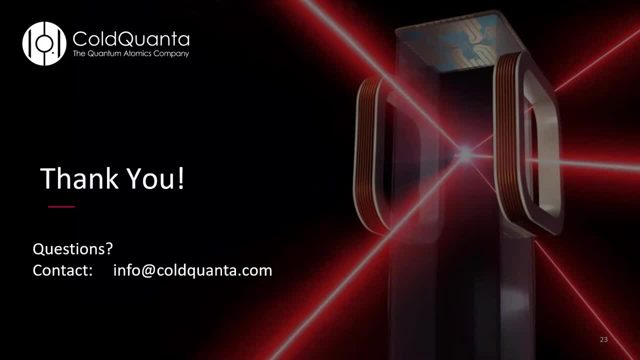 orientation, from the side, for instance, or from below, In this case, the way the vacuum chamber is configured. when we take these images, after we release the atoms from the trap, they're affected by gravity and so they accelerate downwards in the lab frame, and 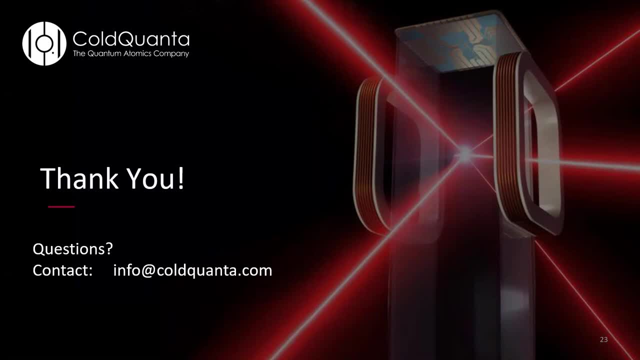 it's just more convenient in most cases to have atoms fall down into vacuum than down into a chip. So in this case we have the objective above it. Okay, great. And then the second question here, which is another triple question actually. 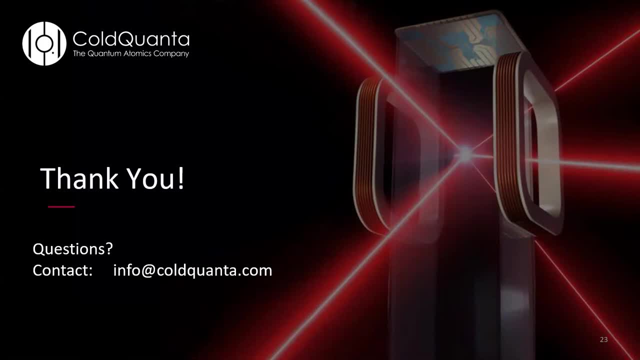 For a shaken lattice gyroscope. where does the self-interfering atom come from? Does it get kicked out of the on-site of the lattice, Or is it introduced externally? And is there only one atom or many? Okay, I'll try to get to all those points. 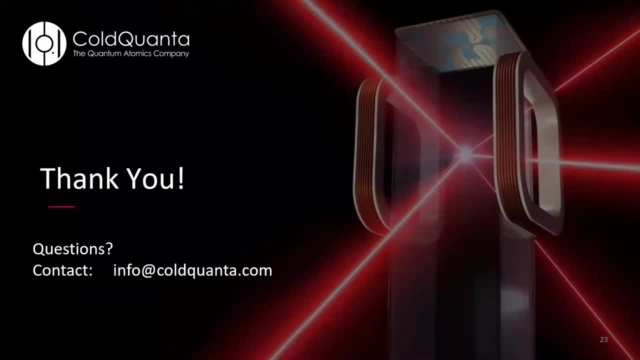 So in the lattice, depending on how you know what the parameters are of the lattice, you can either consider an atom to be localized at a single lattice site or, if it's shallow enough of a potential, you can have it actually delocalized across many lattice sites. and 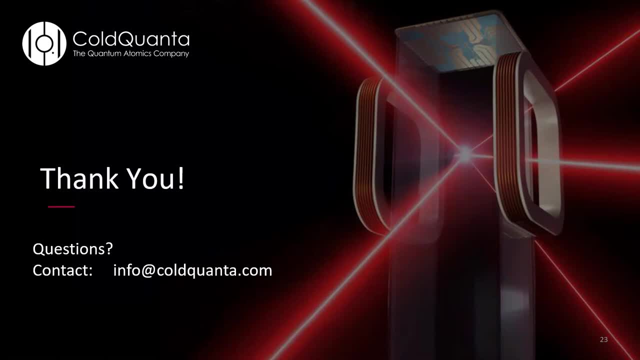 you really have to start thinking in terms of band structure of crystals and how modes transfer or translate in crystals. So rather than having some nice wave function, like it does in a magnetic bowl trap, it has a different type of wave function And this wave function actually can be translating. 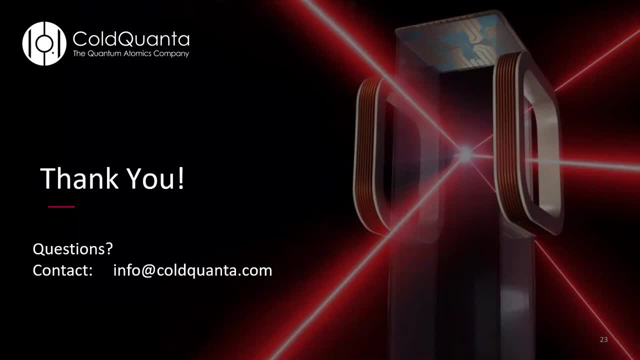 counterpropagating one another, for instance, or coming together back again at the end of some interferometry sequence. So you actually have the wave moving in the lattice trap and the interference comes from multiple waves. who've moved out and maybe come back to reinterfere that I 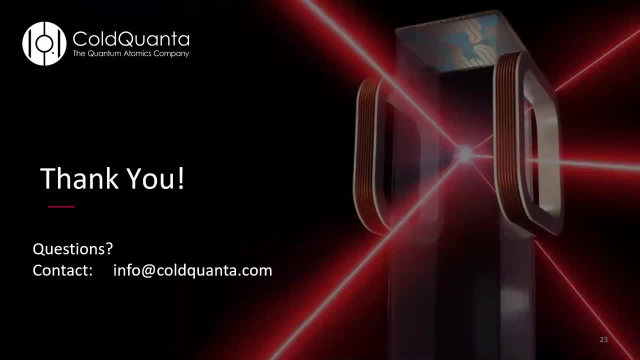 guess in getting to part of your question, it doesn't come from the outside, it's all waves from the inside and then, in this case, for the gyroscope at least, we can consider the case of having numerous atoms. so you have waves that go out and come back after accumulating different amounts of phase. 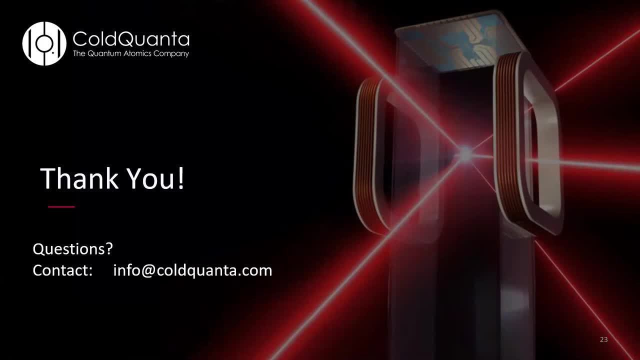 and that phase shift is what gives you a difference in the interference pattern at the end. Okay, and what is the maximum atoms number in BEC? What is this effect and what affects it? So there's a lot of different things that go into both number and temperature of atoms in a condensate and, in particular, 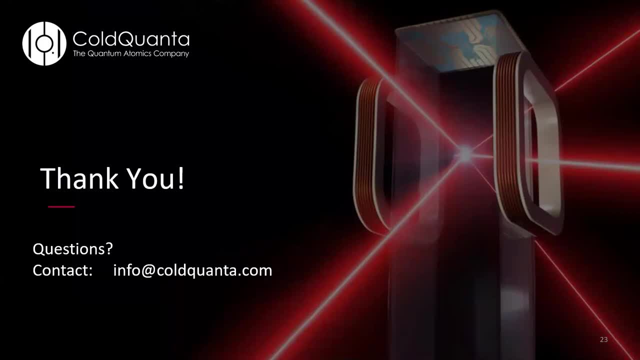 a lot of system parameters like trap frequency are coupled to these thermodynamic quantities of number and temperature and there's no necessary upper bound on the numbers of number of atoms and condensates. typically people try to make larger condensates because it gives you more signal to work with and 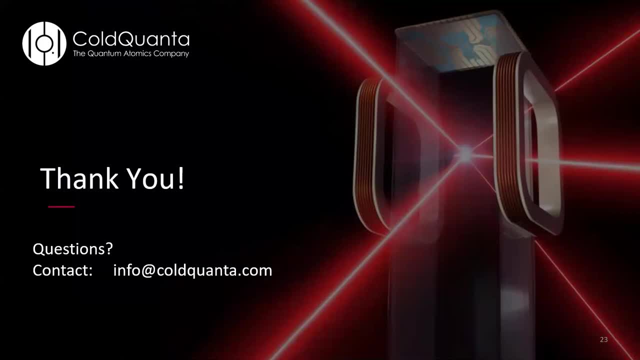 I think there's been recorded cases of millions of atoms in condensate. whether it be 10 million, I'm not sure, but there really is no upper bound. it's really a matter of efficiency and how well your system parameters have done all the way from the beginning, with laser cooling through evaporative. 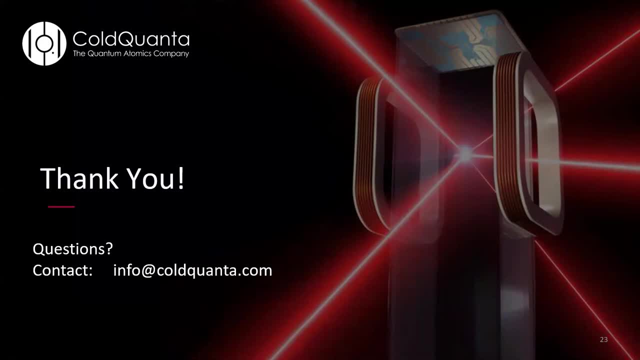 cooling and how efficient you've been with your starting atoms. typically in a MOT you start with something like billions of atoms and at the end you reach the smaller number number of condensed atoms through the fact that you have to kick some out to cool the atoms. okay, thank you. there are a couple of 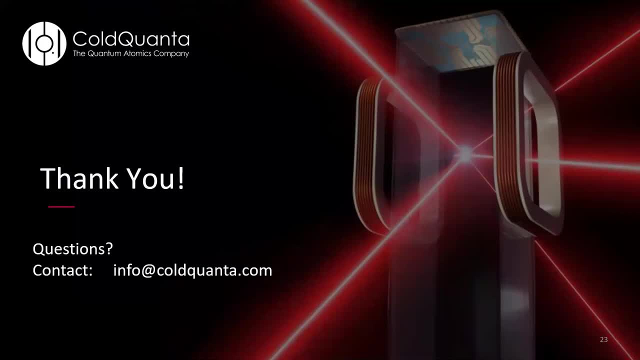 questions about the service itself. so a lot of that work to our listeners is in progress, so we're not going to really answer those at this point, so stay tuned. oh, so here's a new question just coming in: Can all of the atoms in a condensate and in a condensate have the same number of atoms? 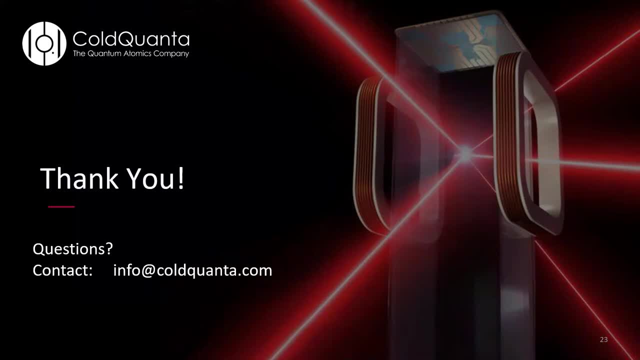 Can all of the atoms in a condensate have the same number of atoms? Can all of the atoms in a condensate have the same number of atoms? Albert accommodate multiple atomic species, ie alkali atoms also, if I wanted to do an EIT experiment, for example, can Albert accommodate RF source input? 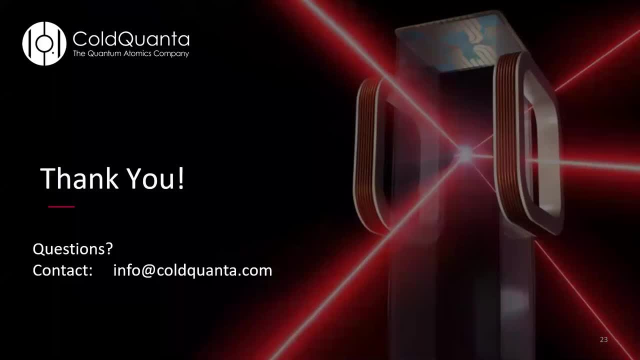 Sure, yeah, these are all uh parts of the discussion we want to have with uh folks like you on this webinar. uh, we have done systems with multiple species. In fact, the one on the International Space Station is multiple-species based, So that's open for discussion. 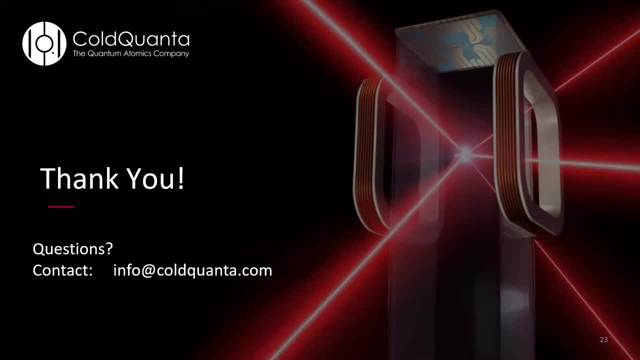 Initially, we'll most likely start with rubidium only. That's what the system that we're working with, CU Boulder has currently available, But we expect to make numerous of these machines and we certainly agree with you that it'd be interesting to do not only alkali but alkaline earth metals. 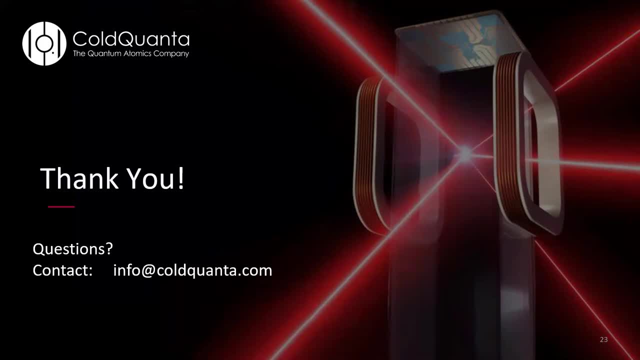 So that's certainly something we'll discuss and we can maybe have some sort of popular poll to decide what we put in there. And you asked about EIT also. So Coal Quanta is quite familiar with EIT and we currently do EIT experiments in this. 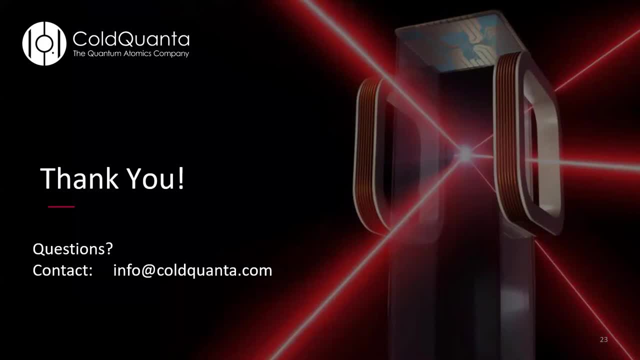 type of system, Or at least one similar to it. So we can certainly consider putting in things like RF horns, antennas et cetera and try to mitigate things like unwanted reflections. So thank you for the question. Okay, For quantum computing applications using identical atoms means identical qubits. 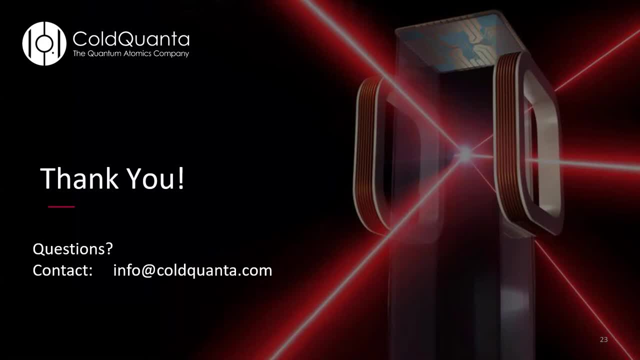 But how carefully do you have to control the optical potential field in order to make sure that the wryberg wave functions of the many atoms are also identical? Okay, So that's getting quite technical and a little bit outside of my wheelhouse, And we have folks here at Coal Quanta who would know exactly how to answer your question. 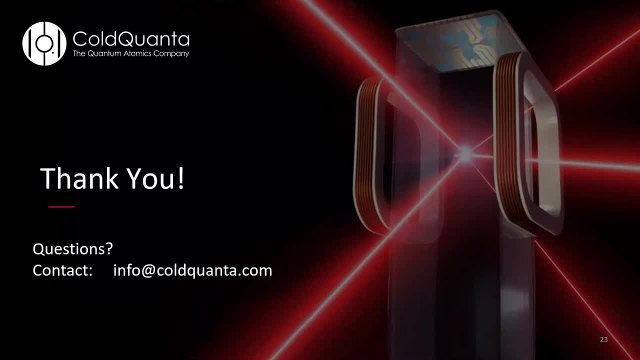 Unfortunately I'm not one of them, So I encourage you to stay tuned for when we'll have a deeper discussion on our neutral atom quantum computing system And you can ask. I'm a true expert at that question. Okay, For the modulation of the lattice beams, is the beam stationary, ie adjusting phase? 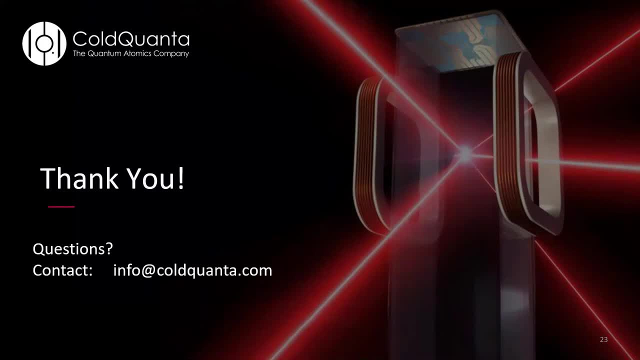 amplitude frequency, or are you actually stirring the beam? Yeah, Okay, Good question. So the K vector, Let's say the K vector, direction does not change. Perhaps it could, but that would get a little convoluted, I imagine. 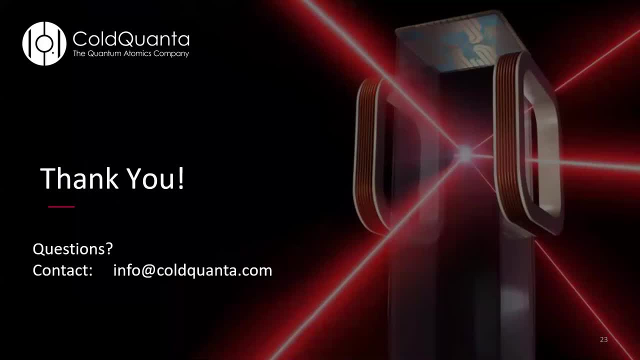 In fact, like you said in the first part of your question, We can control the amplitude and the phase or the frequency or one of these other sorts of characteristics which changes how it. You can think about it a little bit like diffracting the atoms in a grating 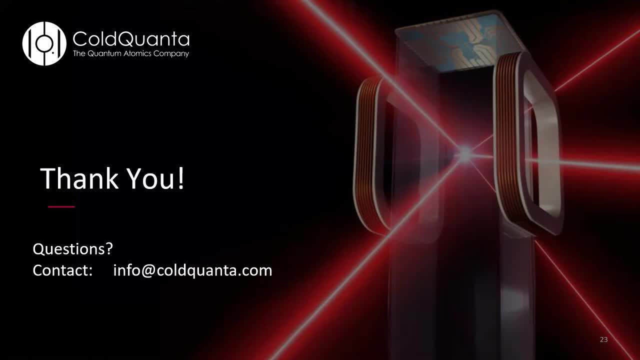 So you're controlling that diffraction pattern? Great Well, thank you. So that's going to be the end of our questions today. We thank you all for joining us And, Seth, thank you for all the information And again, regarding the specifics of when we will launch the access publicly via remote. 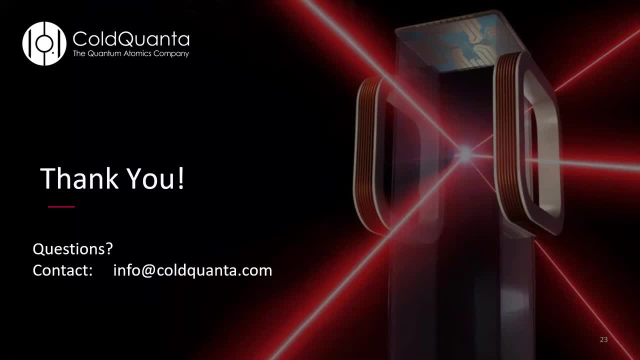 access via the cloud. stay tuned. We will have some marketing around that and information will be available on our website. So stay tuned for that And thank you so much. Our next webinar will be on June 11th, and watch for the invite. 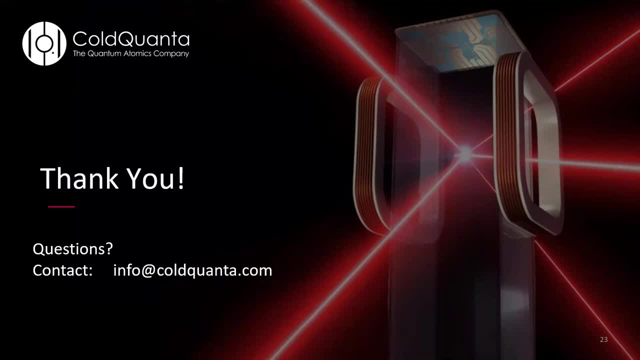 Everyone have a great day, Bye, Bye.